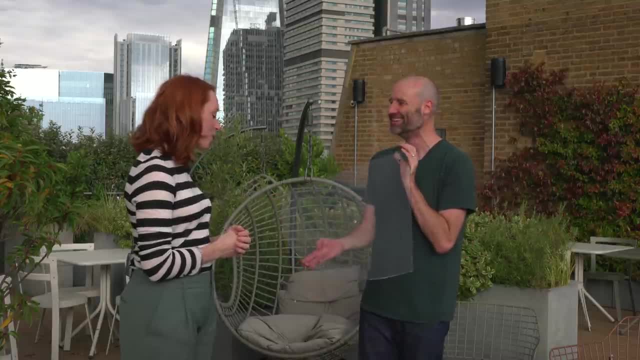 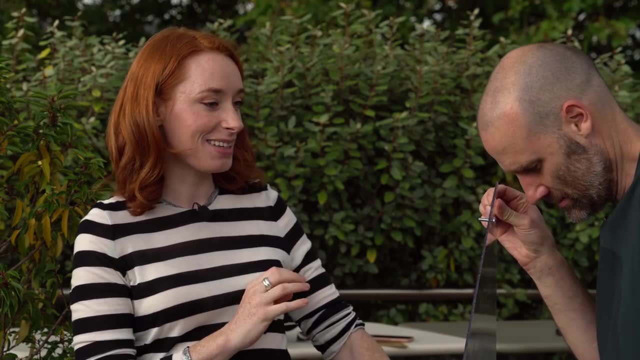 It melted. I had to file it off this morning Also. I mean, I accept what you're saying. You want to do it the original way. You want to do it the Albaruni way. I don't think they had clear Perspex in a thousand years ago. 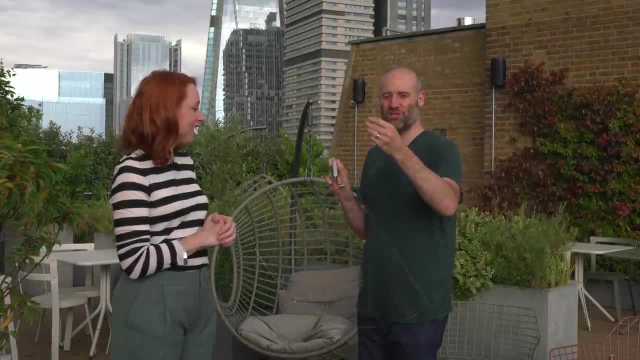 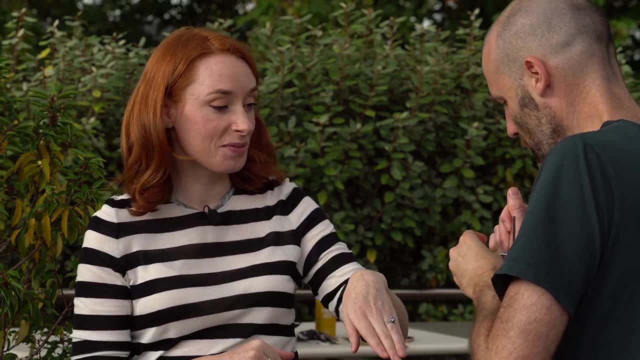 Well, my bronze machining skills are woefully inadequate for this task, So I bought Perspex and I Did a quarter of the job. Did a quarter of the job. It's all you need. I live streamed it, by the way. 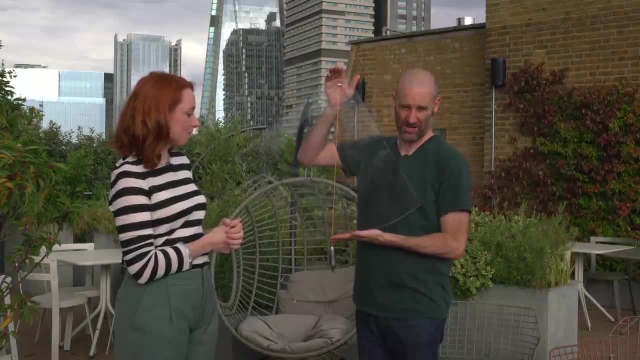 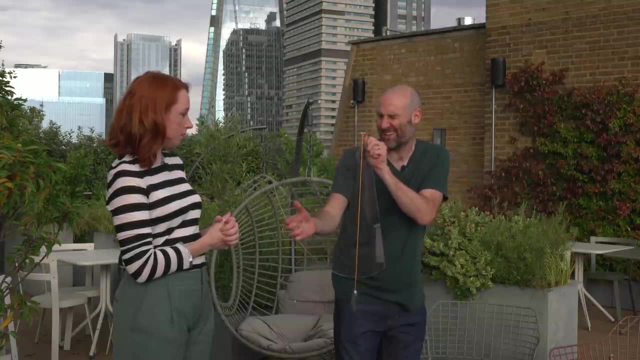 I'll link to it in the description. I honestly made this from scratch with a compass And a straight edge, And it's not bad. So instead of using your inclinometer, I'm going to point this at the horizon like that. 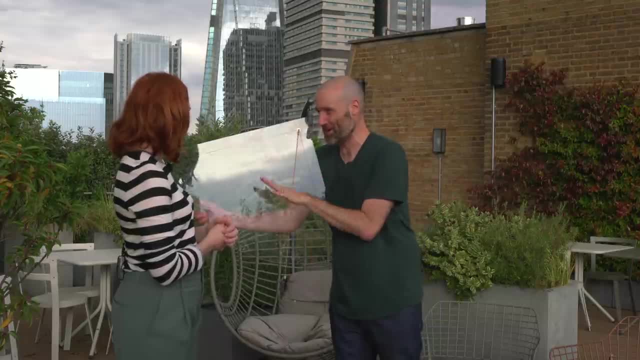 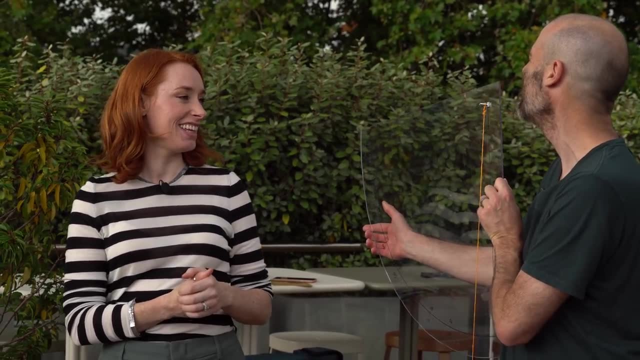 And then I read off. I might need your help. if I'm being honest, Did Albaruni have an assistant, I assume. so It's a real two-person job. So I'll line up like this And then, without moving it, you can either hold it or you can look down there. 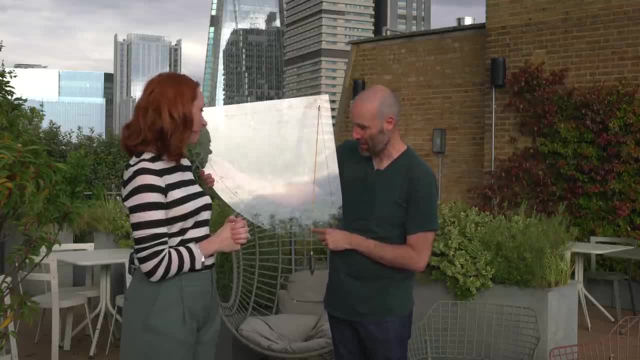 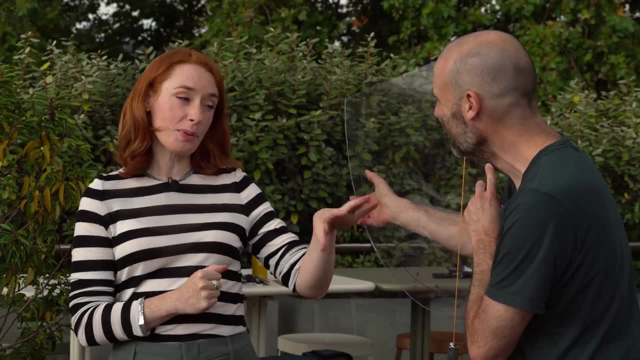 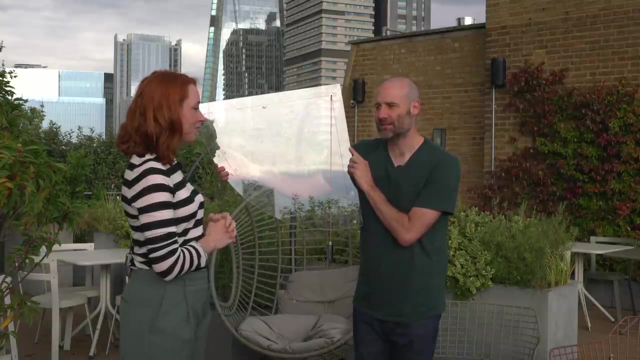 I've only marked to the nearest degree. Sure, But you've just got to estimate what percentage through. Okay, So okay, But we probably can get a reasonable estimate for the actual radius of the Earth just using this and the shards. What would we count as a success? 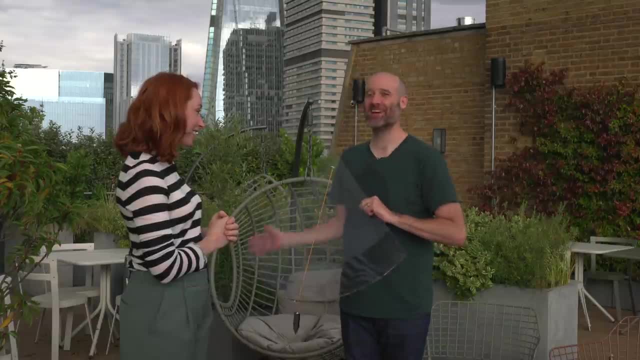 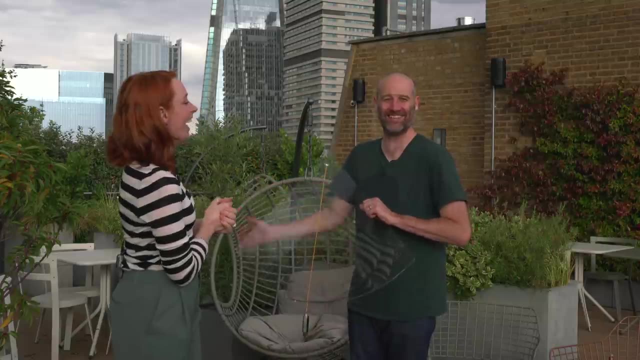 Within 1,000 kilometers. Really, I was thinking if it's not negative, I'll be Anything between 10 and a million. I will consider a success using this. I think that's generous Within 1,000.. All right, 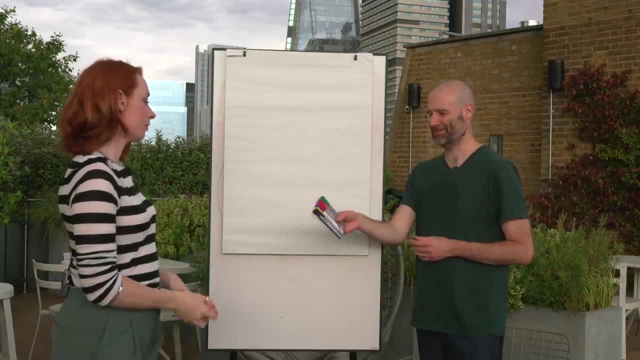 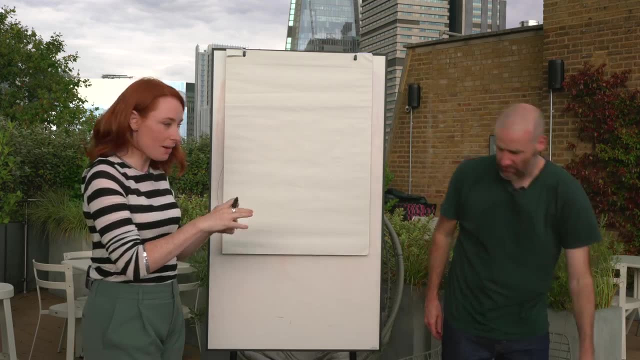 Thank you, Bye, Bye, Bye. Let's see the triangles. I think this is kind of a mad idea that you could measure the radius of the Earth, Yeah, with just a couple of triangles and a mountain and a bronze astrolabe. 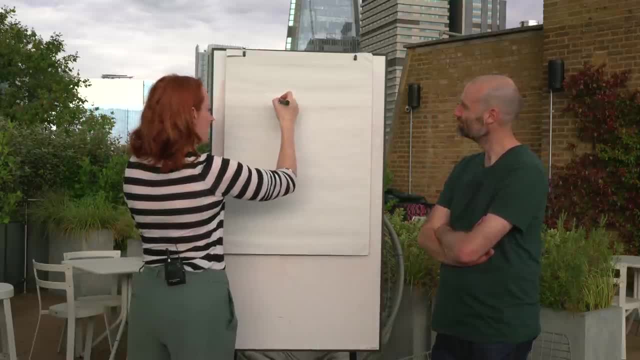 Okay, So let's say you've got the Earth like this. My circle drawing isn't. It's been a while. That is Absolutely terrible. That is oblate, I'll give you that. I mean, the scale is about to go very wrong. 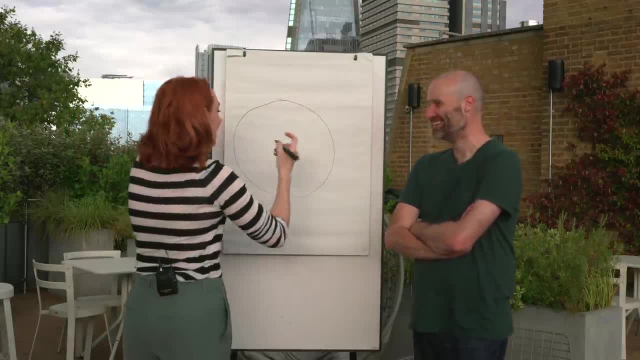 Okay, So say, you've got a mountain here, Yep, Or the shard Gotcha, Okay Now, the center of the Earth is this: This is the center of the Earth. This is the center of the Earth. This is the center of the Earth. 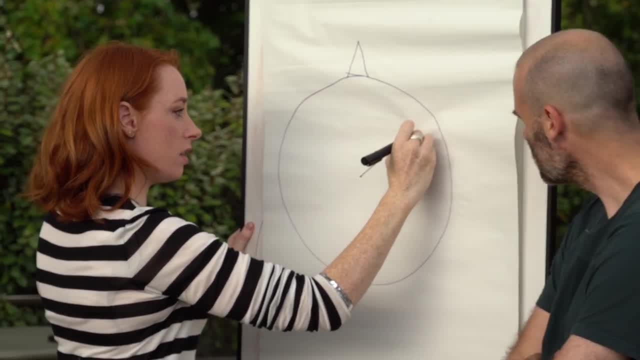 Now, the center of the Earth is right about here, Yep, So this: I'm just going to assume the Earth is spherical for a moment here. I'm okay with that. So this is what you want, right? You want the radius of the Earth there. 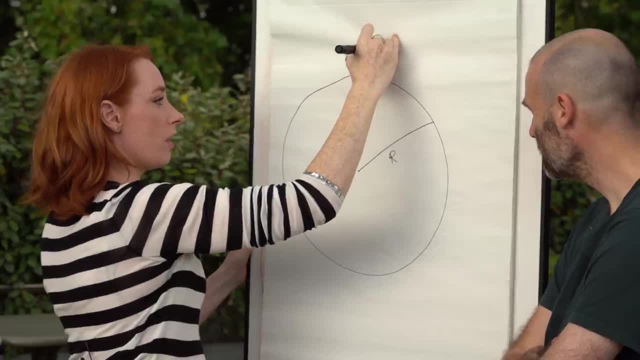 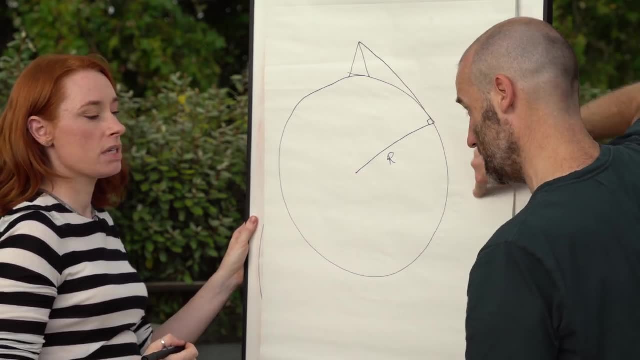 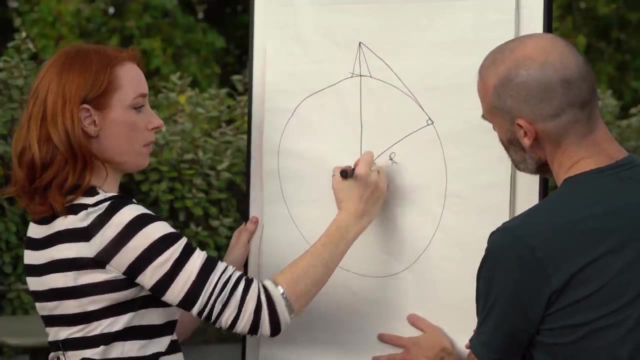 Yep, Okay. Now if you draw yourself a nice right-angle triangle here- So this is you looking at the horizon, Exactly which is tangent to the surface of the Earth, Exactly right Gotcha- Then you can make this right-angle triangle that goes through the top of that mountain. 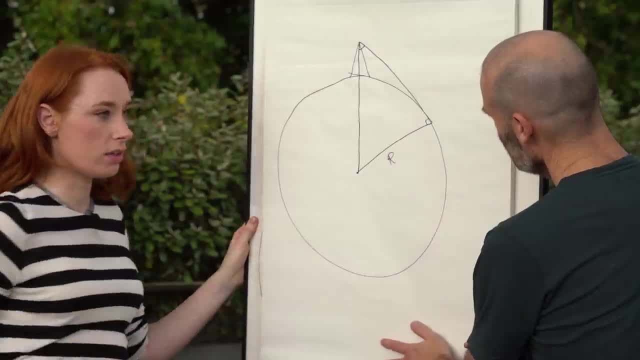 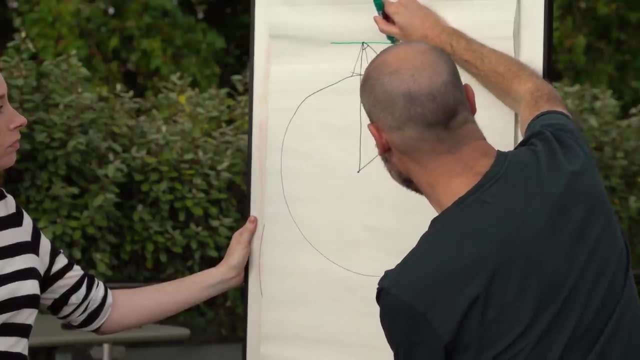 Yep, Now, this angle here is something that you can measure right. It's the angle, Oh gotcha. So we're kind of We're going to measure compared to the horizon. So looking straight out would be this direction. 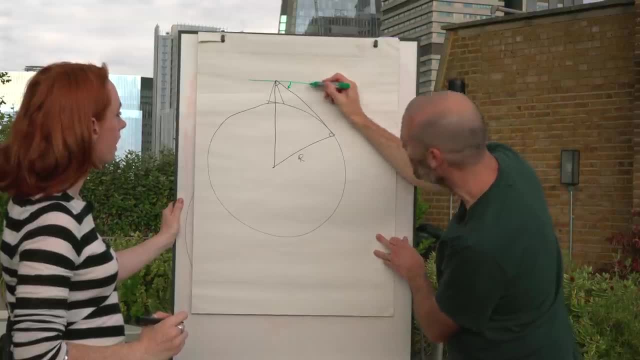 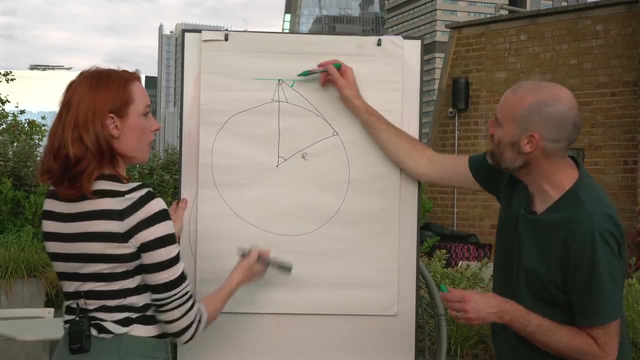 Yep, And then we're going to measure how far down to there Exactly. But that's a right angle, Yep, So the difference will give us that little angle in there, Yeah, Yeah, Or effectively, you do this angle in here as well. 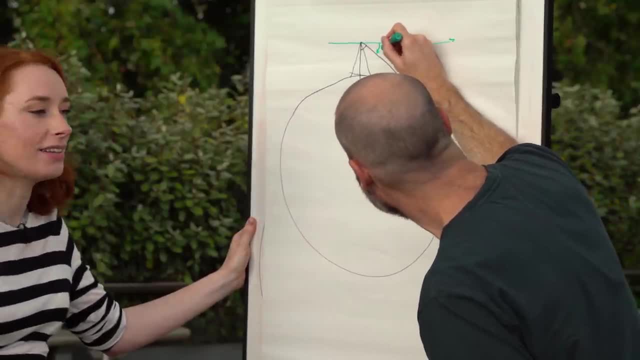 Oh yeah, Yeah, because that angle there, if that was, Let's call it C, Call it C C. Yeah, you're looking at it, Then that there is C. Yeah, Perfect, Gotcha, Now this is a right-angle triangle, right. 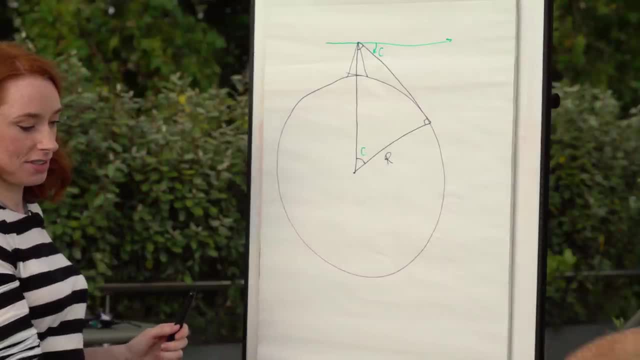 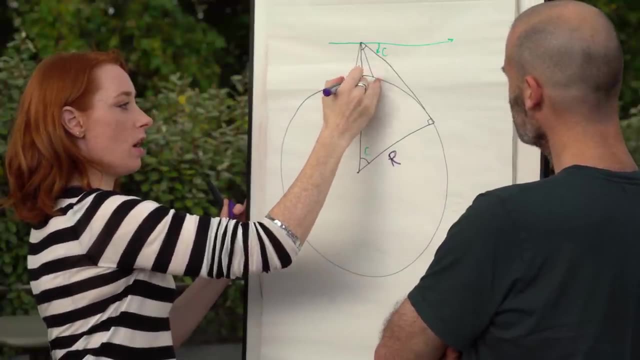 So we're going to measure the distance here. Can I have another color pen? Yeah, sure, Let's go purple, Beautiful, Okay. So R is what we want. We want to get R, But this here is also R. Up to there is R. 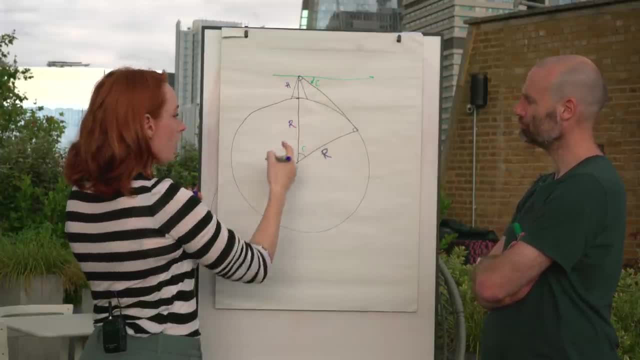 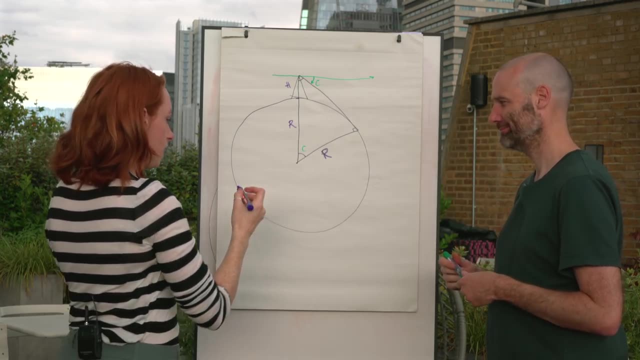 Yep, And this here. let's call it H H Gotcha. So now you've got a right-angle triangle. One side is R plus H, Yep, And you've got an angle that you can measure, and the other side is R. So it's really simple. 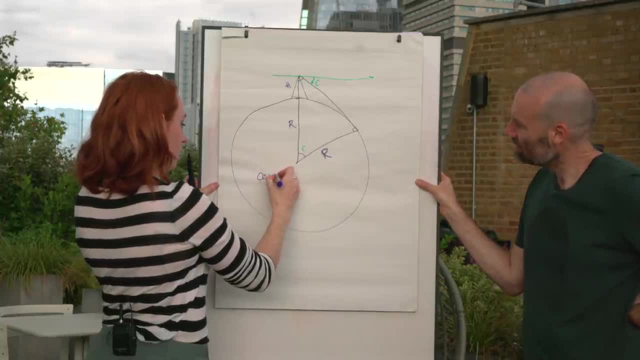 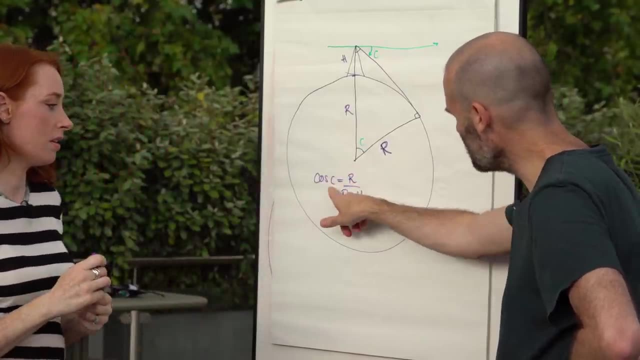 right, It's just cos. C equals R. Okay, So R plus H, We measure C. Yep, We need to know H. To give us R, We get R. Yeah, So we do need to know the height of the charge. 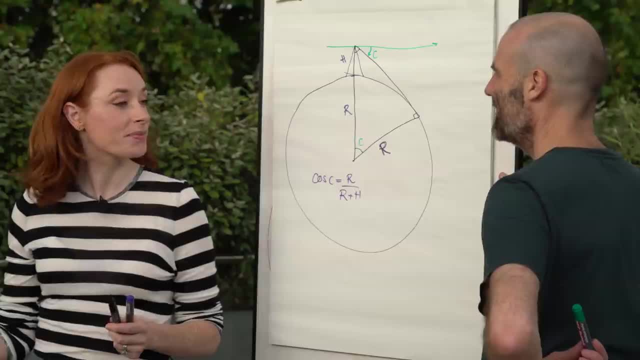 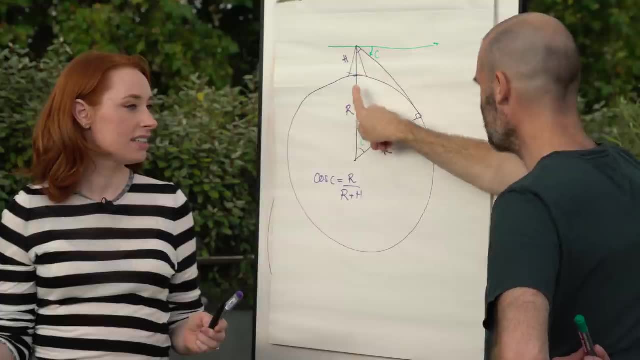 Okay, But that's okay because I can just look it up. Oh, Whoa, whoa, whoa, whoa. Al Baruni did not look it up. He used a mountain, Yeah, And he must have calculated the height of the mountain. 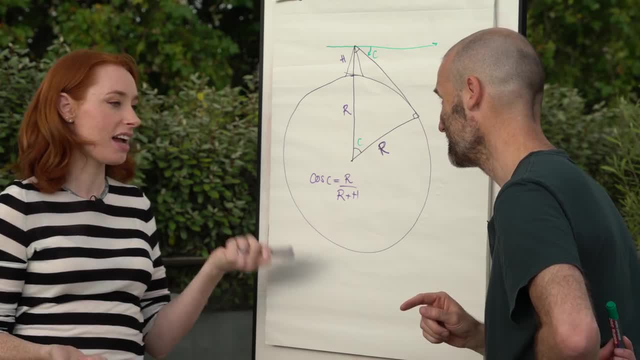 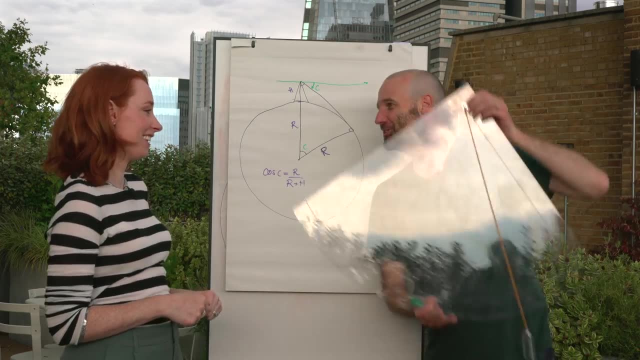 Yeah, Which is in your book. Yeah, I mean, you can use triangles again to calculate the height of the mountain, but I don't want to be here all day. No, no, We've got to do that. I didn't handcraft this to look up the height on Wikipedia. 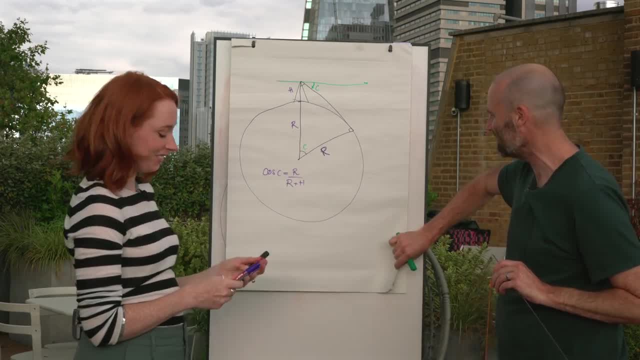 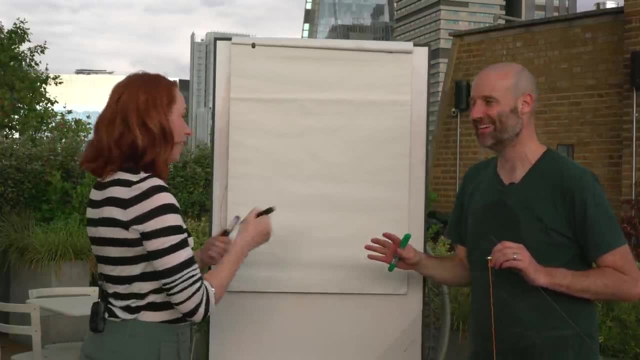 Right, Okay. So break down these triangles for us. Here we go. All right, So you want to work out the height of the shard as well? Yeah, yeah, yeah, Okay. All right, We're doing the whole thing. 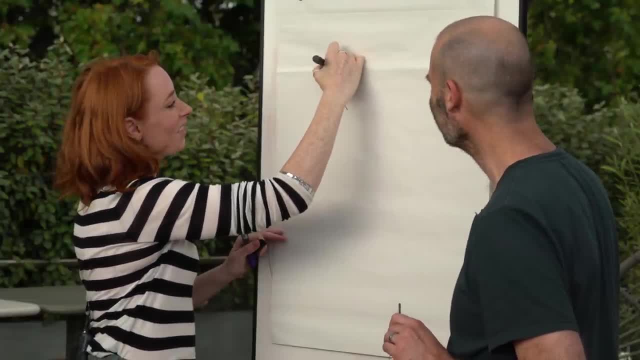 Okay, okay, okay, Fine, All right. So here's the shard. then Come on. I grew a beard for this and everything, And a very impressive one it is too, Thank you. So here's the height Going old school. 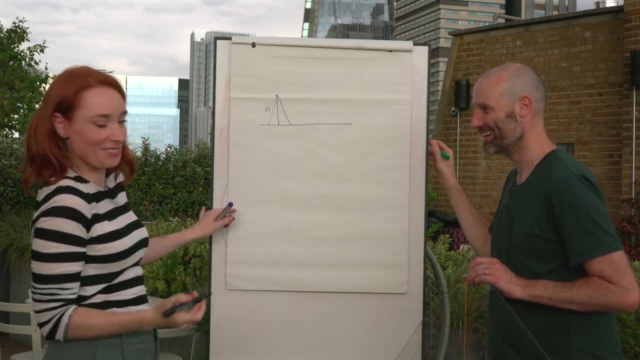 This is the shard. Yep, It's close enough to the shard that the earth can be flat, Gotcha. So now, Oh, yeah, yeah, yeah, I'm happy to assume that The way that you can do it. I've retracted now. 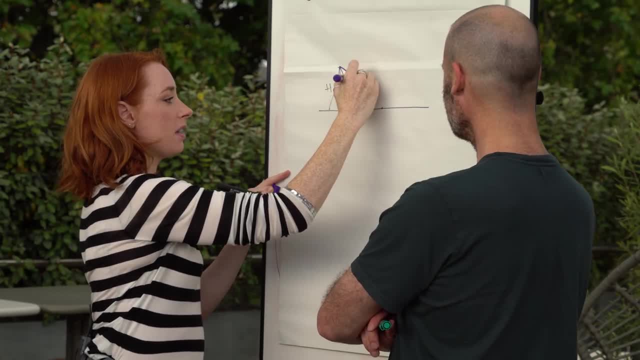 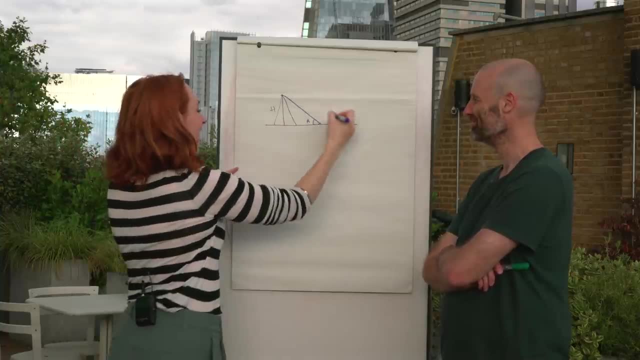 is from a reasonable distance away, say here: Yep, we can look up Gotcha at the shard, measure that angle. Hey, Wow, I'm going all over the place with the letters here, Yeah, And then we'll go a little bit further away and we'll measure it again. 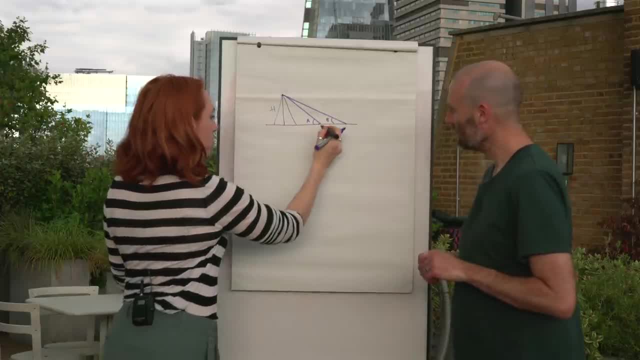 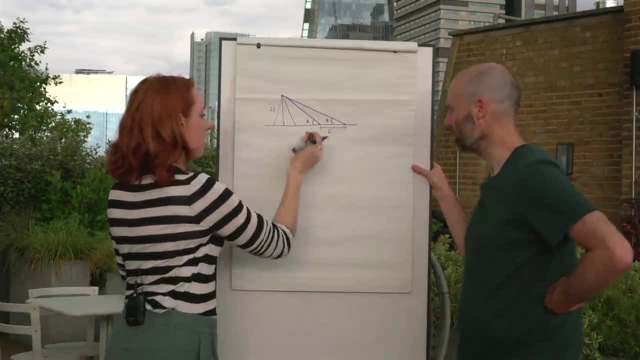 B, And then, as long as we know this distance here, maybe we'll get it, Maybe we'll do like 100 meters or so. Yep, Let's call that D, Call that D for distance. Yep, Then you can use just simple trigonometry. 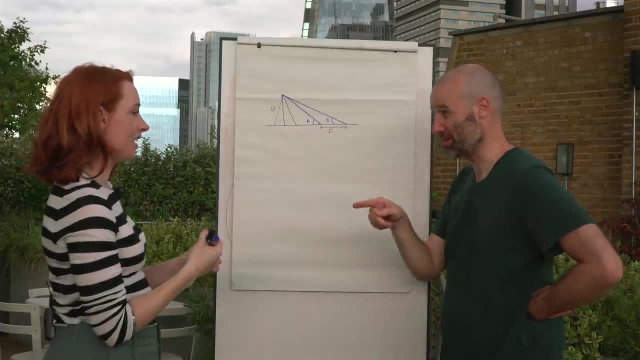 to get the height over here, to get the height over there. So that's what we're going to do. We're going to go out in the streets of London. Yeah, I'm going to measure an angle here while you're looking it up online. 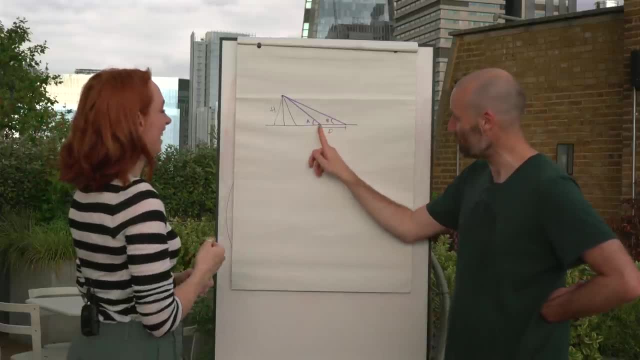 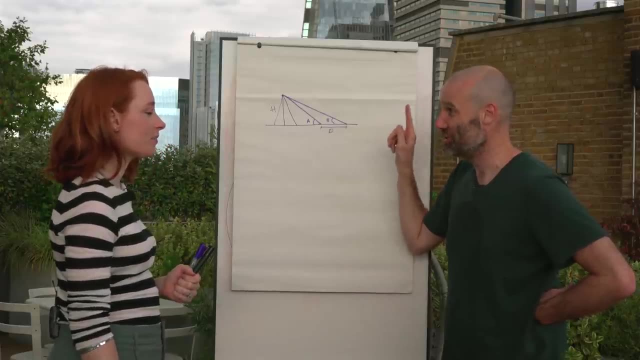 Actually, I'm going to need your help with the measurement. Then I'm going to pace out D. Have you not got a meter stick? Well, Al Baruni did it using cubits, Which is like the measurement of your arm. Yeah, yeah. 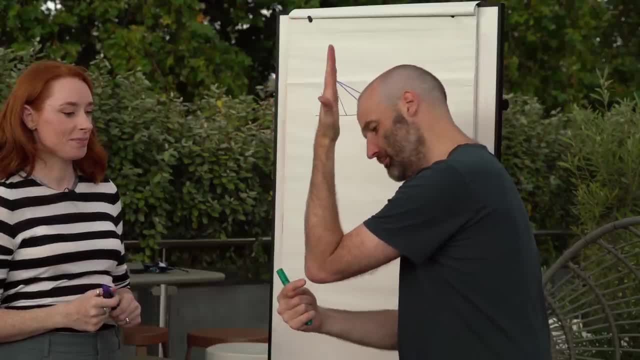 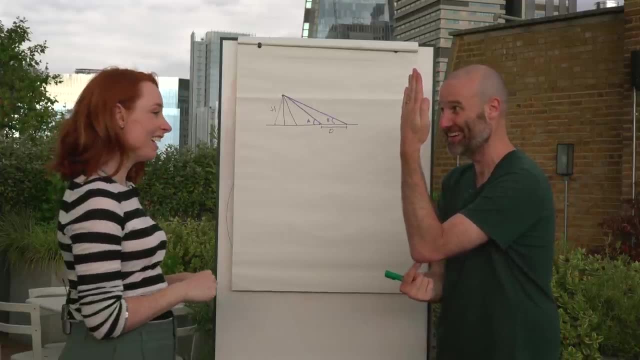 To the middle finger right, Mm-hmm. And so I'm going to use my personal cubit, which happens to be exactly half a meter to the nearest whole millimeter. You're going to go on the floor of the streets of London like this: 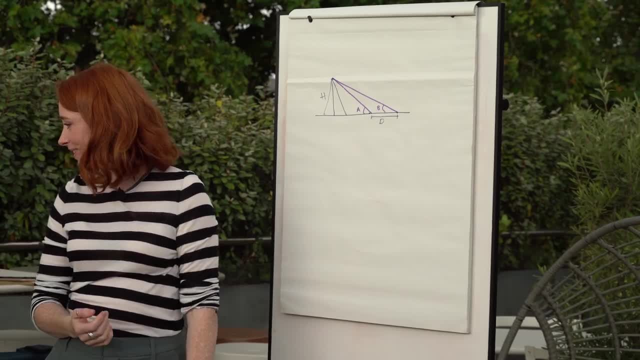 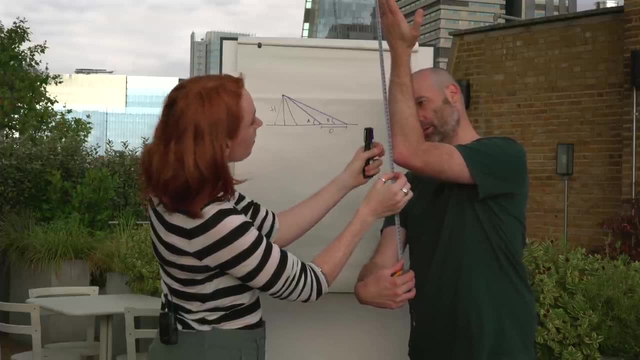 Yeah, No, hang on, Wait, Just so we're clear on this. Here Can you read off? Yeah, Read off a map, cubit. What is it A map? Here's a half. Go on and stretch it fully. 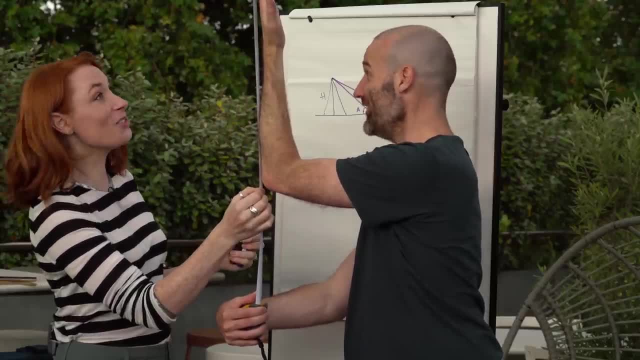 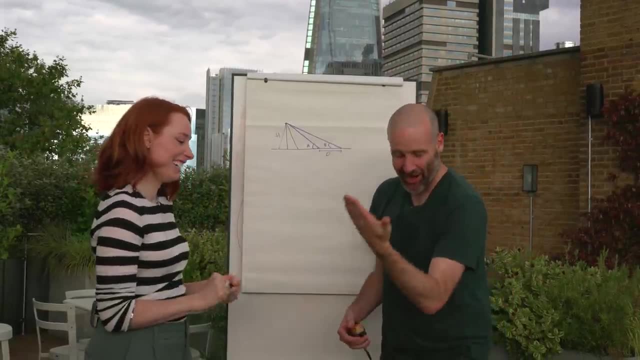 I'm sorry, Yep, Stretch it fully. Yep, 50 centimeters, It's half a meter Built for maths. That's how I'm described, Right? But I'm not going to go along the streets of London pacing them out. 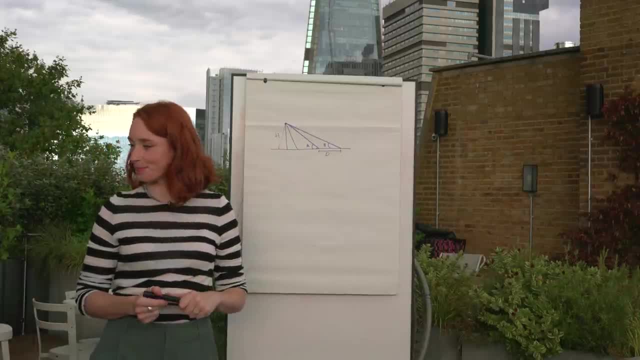 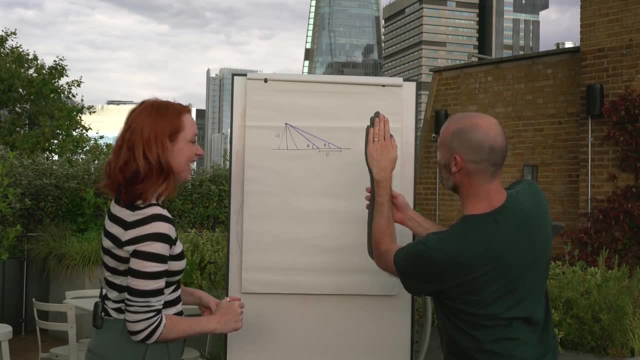 So what I've done? I've made two official Parker cubits Right, And so I traced around my arm. There's one that this I did, each one Right. I'm going to stick these to the bottom of my shoes. 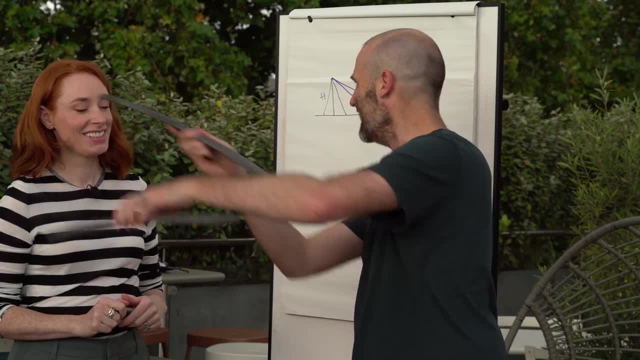 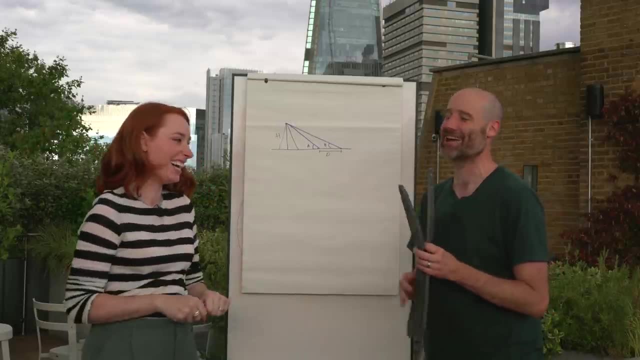 Sure Right, And then I'm going to pace out. Do I have to be with you? Do I have to be with you in the street while you're doing this? Don't leave me on my own. Okay, Come on, Okay. 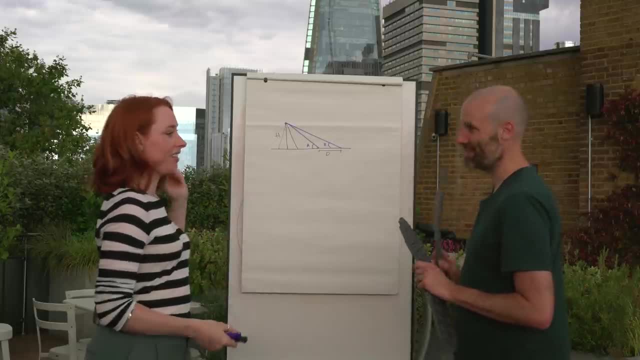 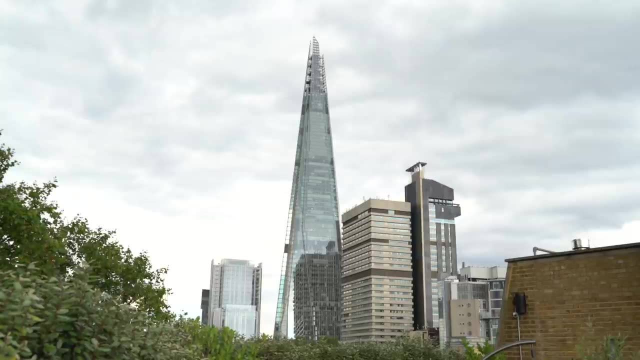 So we're going to go do that and we get the height, Okay, Come back, Work out H and then use that Yep, And then we go up the shot And then, ready to the earth, Done, Let's go. So I'm recording like that angle. 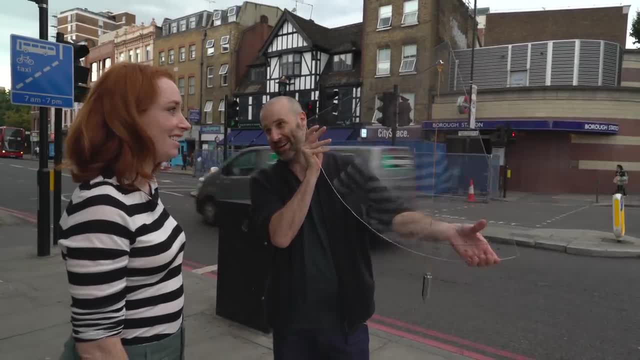 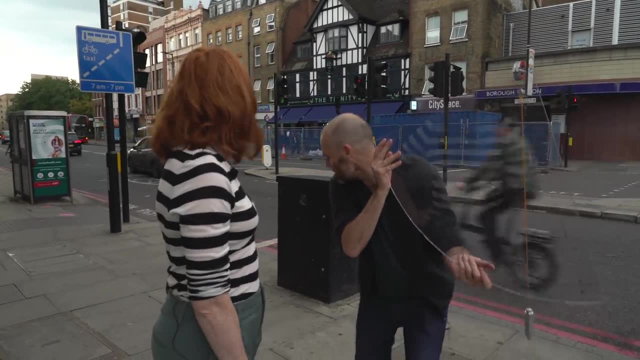 Oh, like this, Right. Okay, So if I point this at the viewing deck, Sure, I'm going to go over here and either hold it or, like, read off the angle. Oh wait, We need to know where this hits the ground, right? 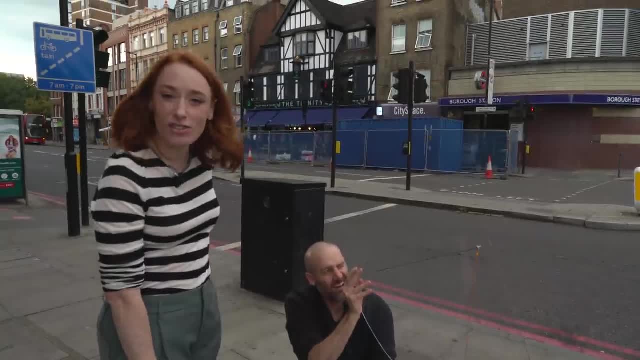 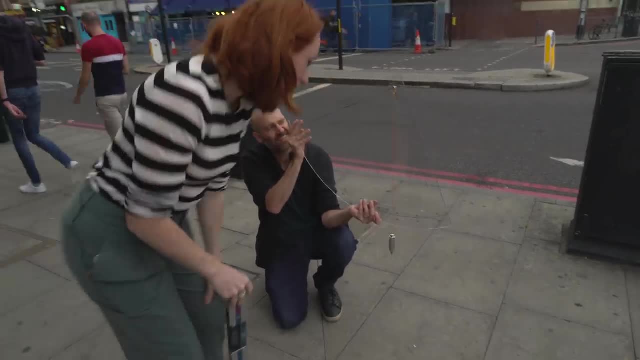 So, if I put it like here, This is not even the second weirdest thing that's happened on this street today. Okay, Okay, Can you come and have a look at the angle? Yeah, Go on, Dr Fry, I need to get around it. 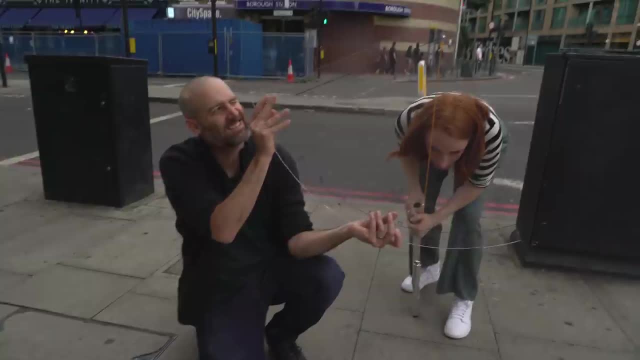 It's actually the best, right? Yeah, I mean, precision is the top priority here. Okay, I'm holding it as still as I can 21.. You can hold it in place or let it. Yeah, I would say that is 23.. 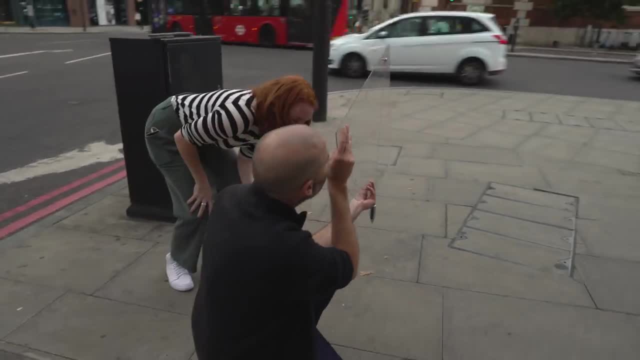 Okay, 23.. Shade under 23.. Are you doing it to a degree? I want it to the nearest 0.1 of a degree. Oh my God. Okay, Well then, stay still. I'm holding it still. 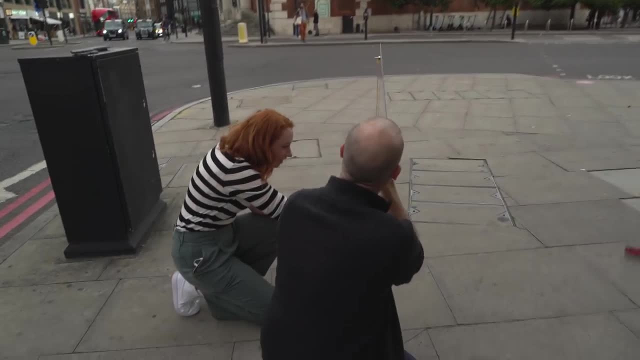 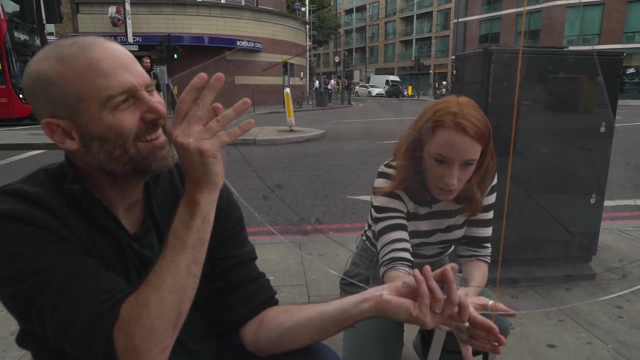 Take the average of it bobbing around. Okay, All right, What do you reckon? 22.9., 22.9., 22.9.. Now We need to Thank you. start taking that for a sec. 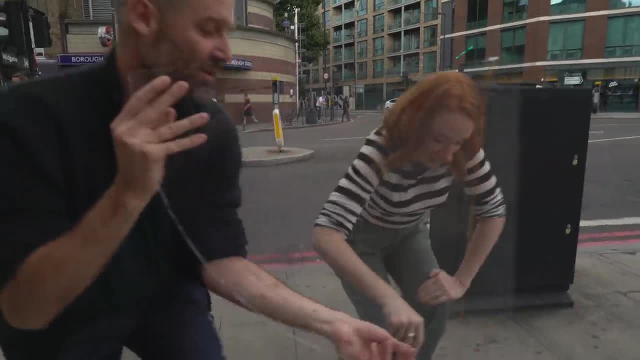 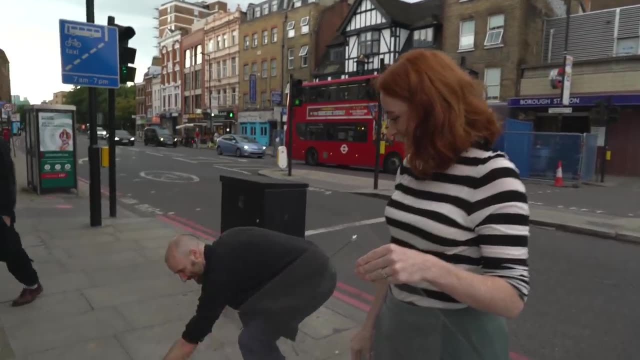 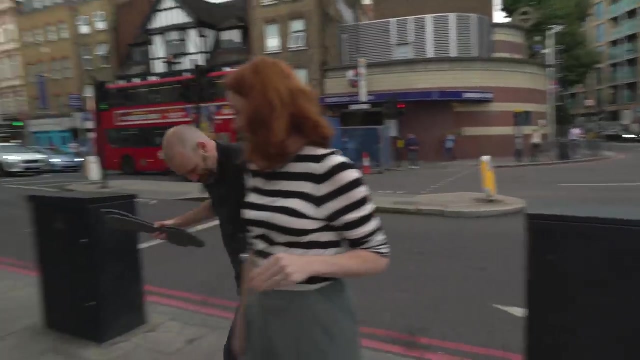 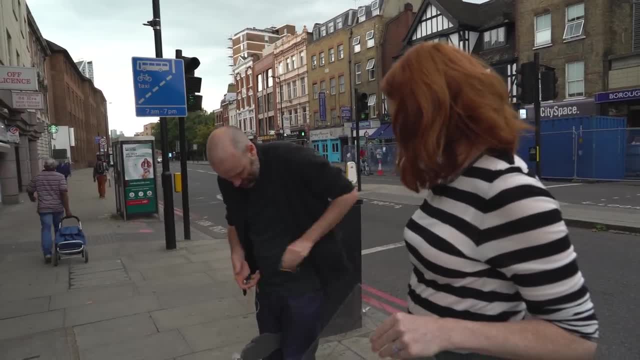 This is so accurate from the ground to now Get these, Okay, And I've brought with me some elastic bands. So what I'm going to do? put my plumb line away. Okay, Here we go. It's a little wonky. 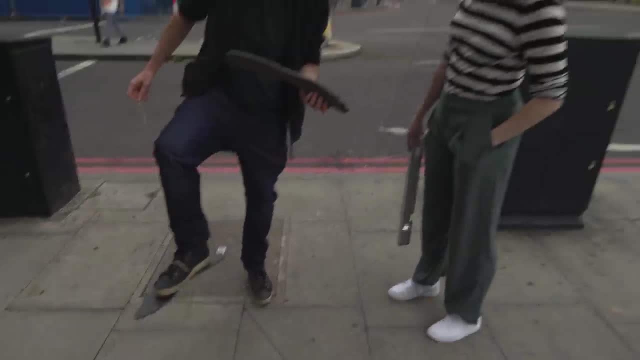 I think Alvaro didn't think That's going to work. I don't think you look this stupid, I don't. Okay, There we are. So now Do you know what it looks like? Look at it. look like. 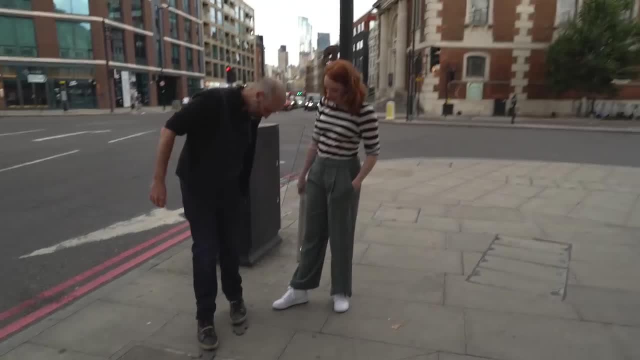 It looks like you're about to walk through sand and protect. Let's do a little walking and pretend to be a dinosaur. It's just like I'm leaving fake dino prints on a beach or something. But your next one's your first step. that's step one. 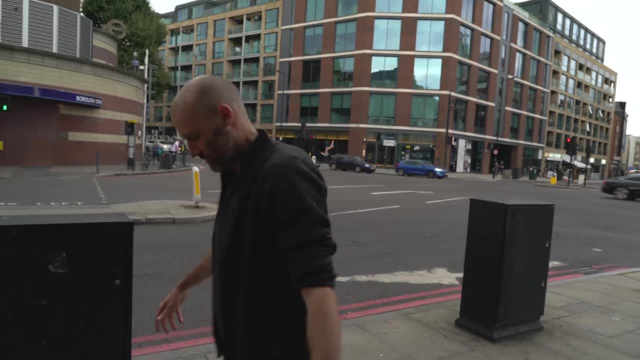 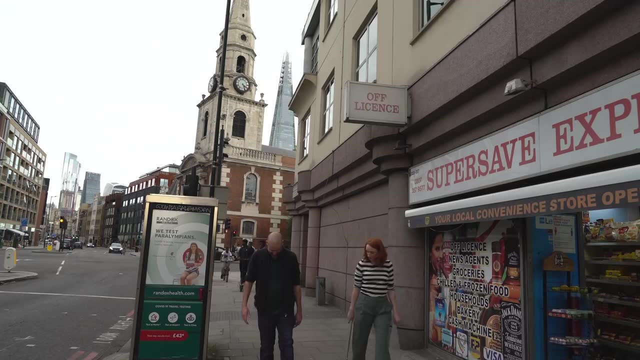 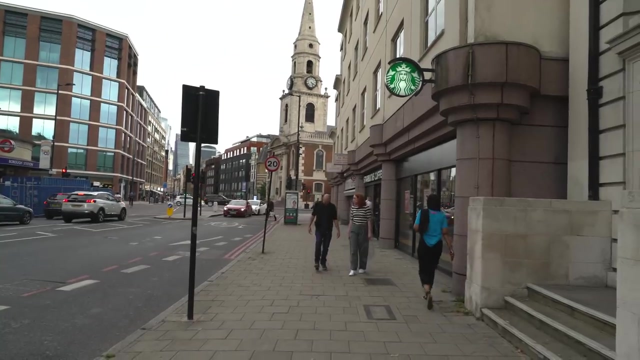 Okay, so one Is that one. Yeah, that's one Zero one. two, three, four- it's already bent- five: 26,, 27,, 28,, 29,, 30. Why am I walking with you? 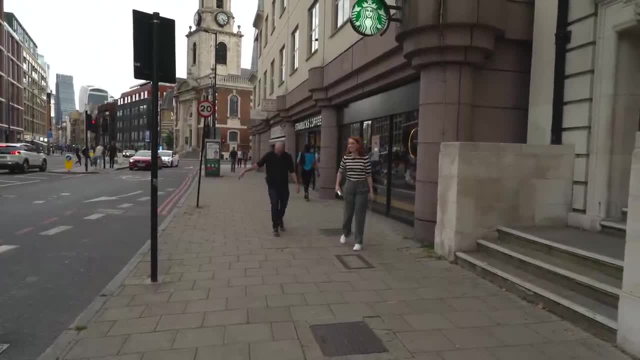 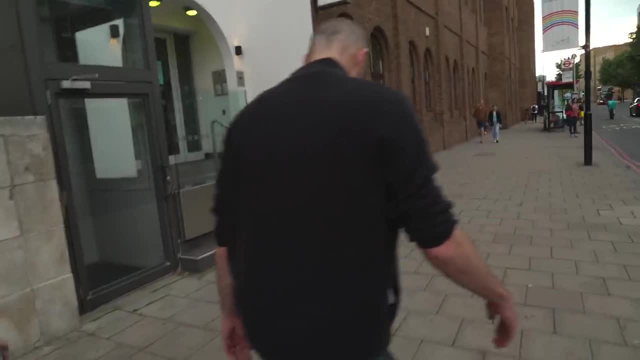 Companionship, you know, mass Solidarity, Solidarity 90.. 90,. oh God, we're not even halfway there. Is that building not going to be blocking our view? No, we can get around and we'll see it. 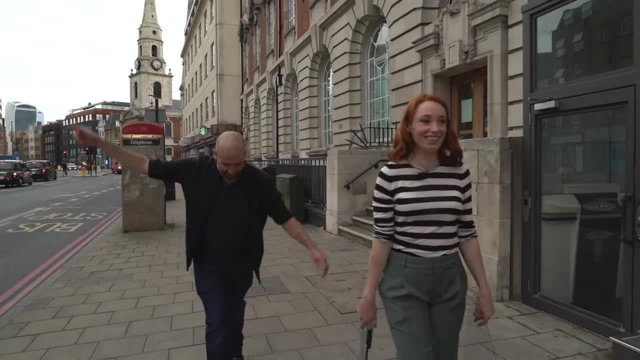 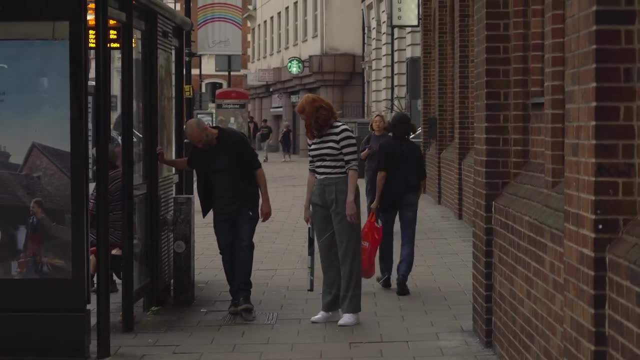 You can see it already up there, see Okay 21,. do I not look like I've thought this through Weirdly? no, Oh no, I cube it 200.. 200 to there, 200 to there. 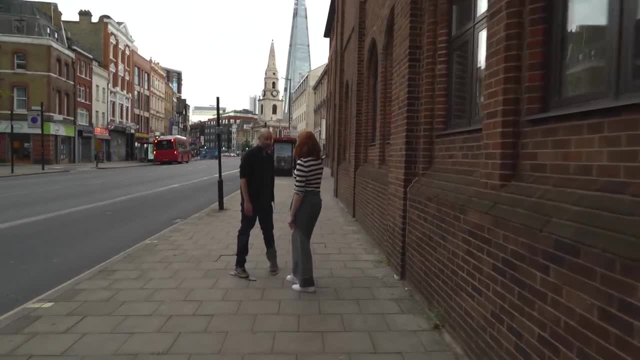 Okay, So do you reckon that's enough? Yeah, it's 100 meters. Yeah, 100 meters. 100 meters, Nice and easy numbers. Should we see if it's a noticeably different angle Angle? Oh, it will be from here. 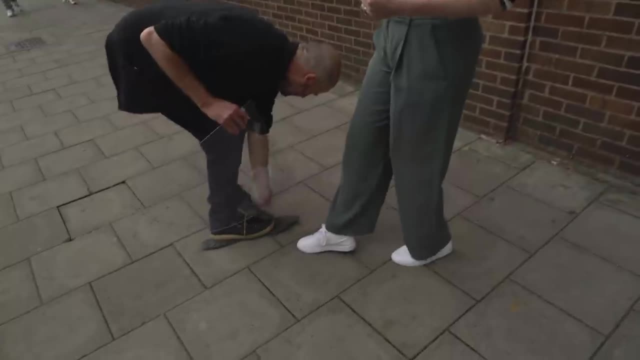 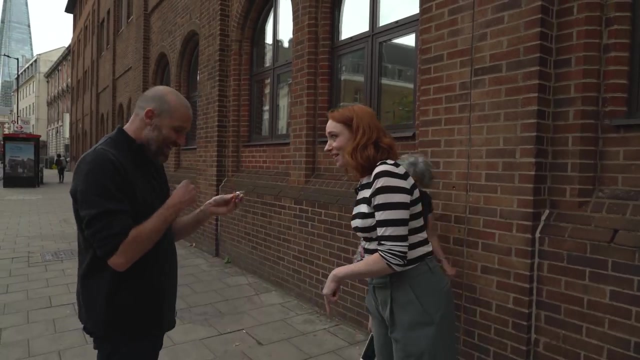 So it's like there, You know what I'm going to do. Yes, I'm just going to snap out there. we go to there. So now you're being precise, Now I'm being. I was precise the whole time. 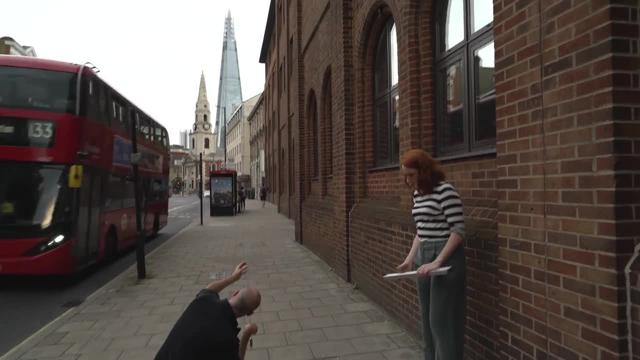 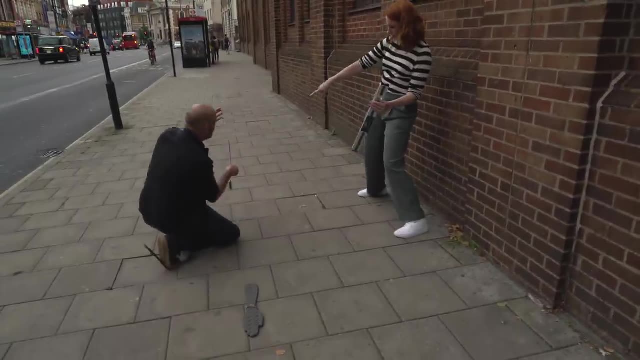 You definitely wasn't. I don't know what you're talking about. How's that? Oh, I'm nowhere near it, am I? No, that's actually pretty good. Maybe move that way half a step. Half a step, that's it, yep. 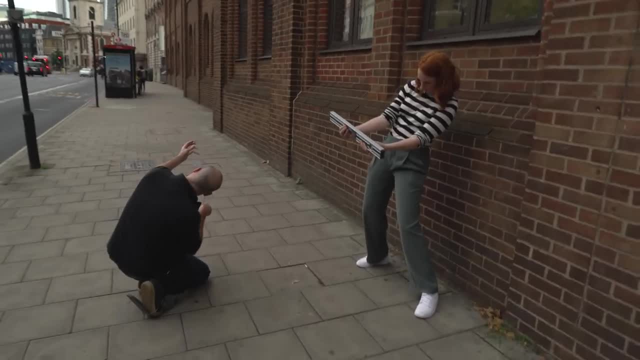 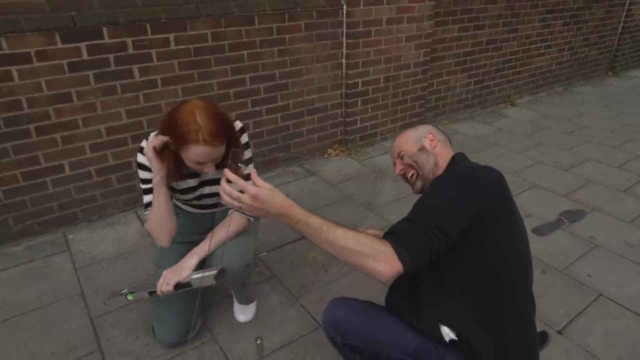 Half a cubit, Half a cubit. Okay, gotcha, That's pretty good, that's pretty good, Okay, okay, what am I on? Okay, Ooh, Oh, don't, don't. I can't hold this and be in suspense. 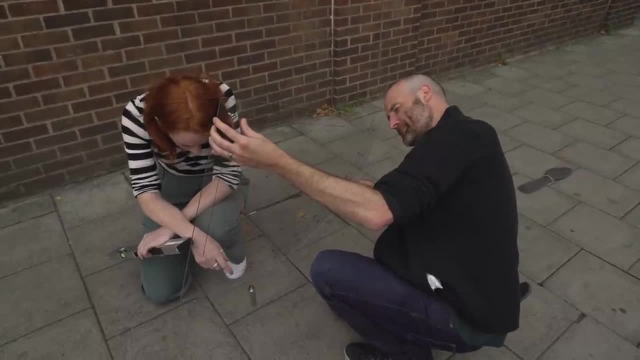 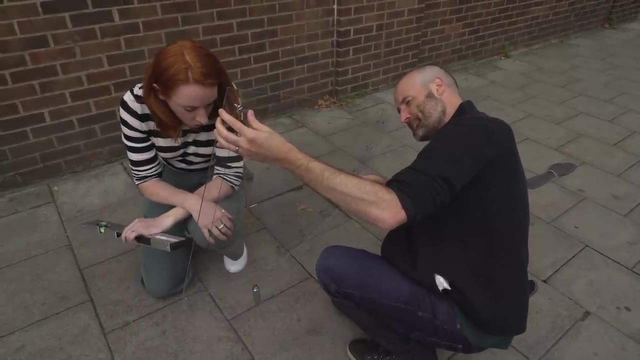 Okay, I reckon that is about 20 point. Do you know? I think it's. it's wibbling around wildly between 19.5 and 20.5.. So let's just go 20. 20. 20.. 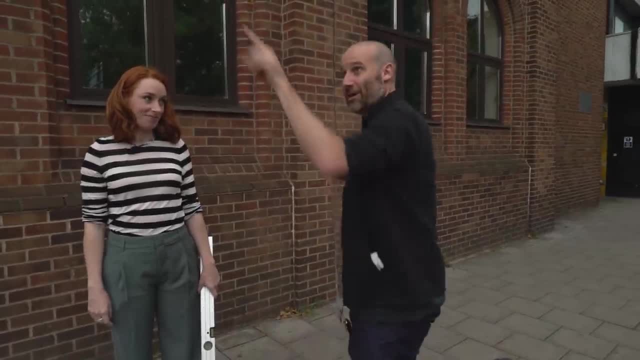 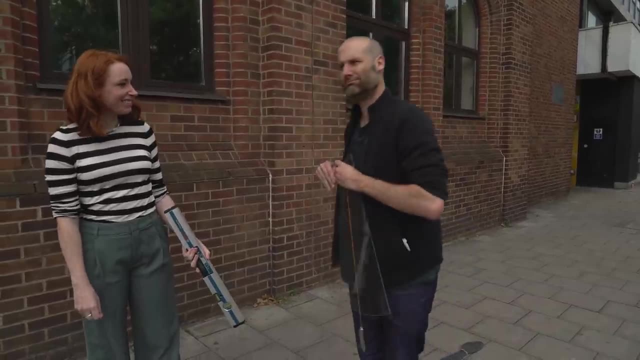 22.9. 20.. Yeah, All right, Now we go to the top. Okay, You're bringing, bringing me. Do you want to double check the distance on the way back with these? Absolutely not, Oh No. 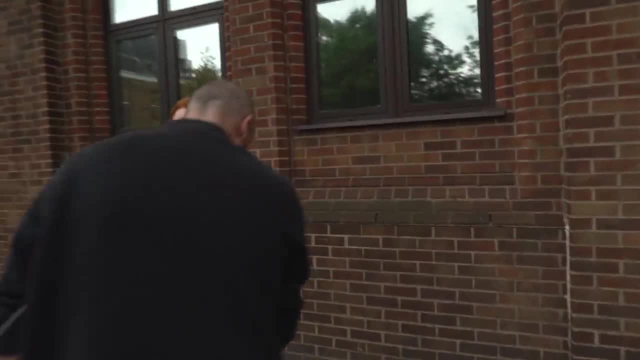 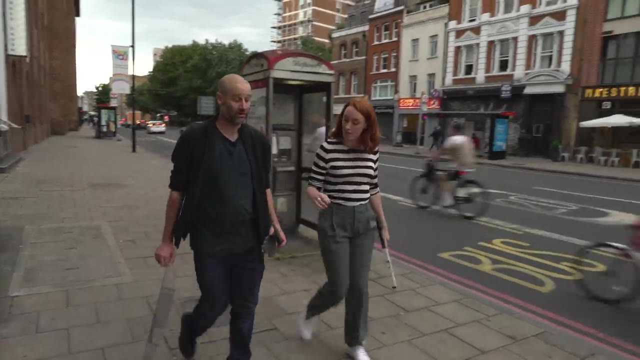 It's weird. It's weird, it's really not. I think. I think once is enough on this occasion. What do you think is going to work? Do you want me to take those? Oh yeah, do you want me to look after them? 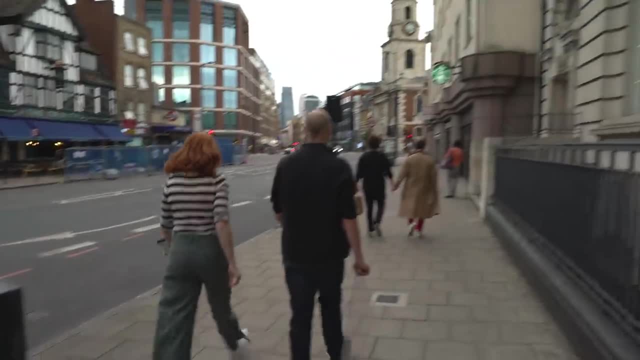 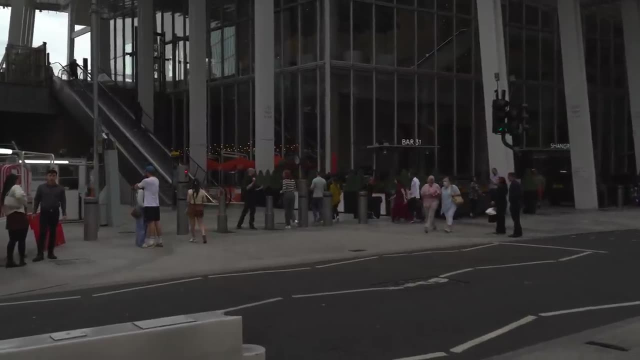 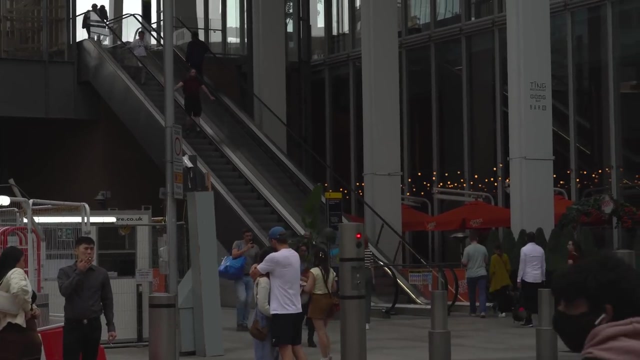 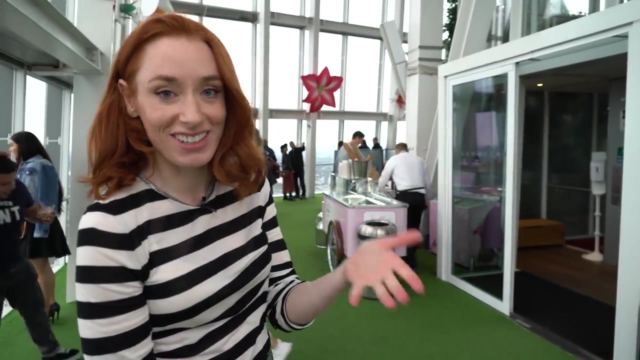 Yeah, sure, sure, sure, That's fine. No worries, It's been a long time making this. Yeah, It's a real labor of love. It's safe now, Don't worry. It's safe now. Matt's not here yet because he obviously took the flight. 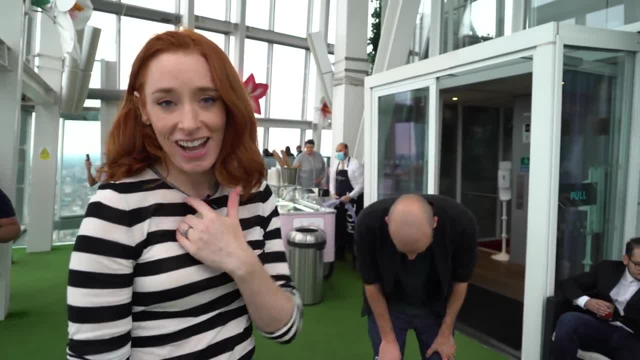 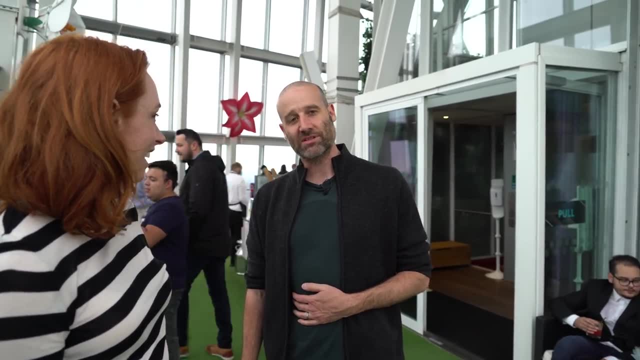 upstairs. all the way up here to the 72nd floor. I took the lift. I've arrived cool, calm and collected. How was it? Oh, it's. what can I say? I'm glad I'm just so in shape. 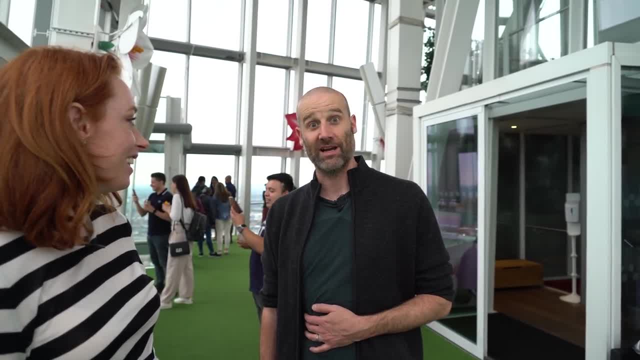 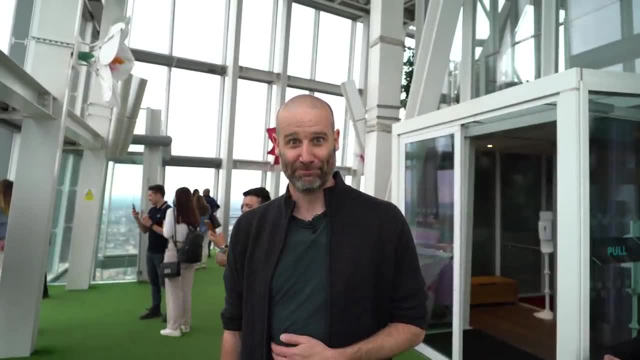 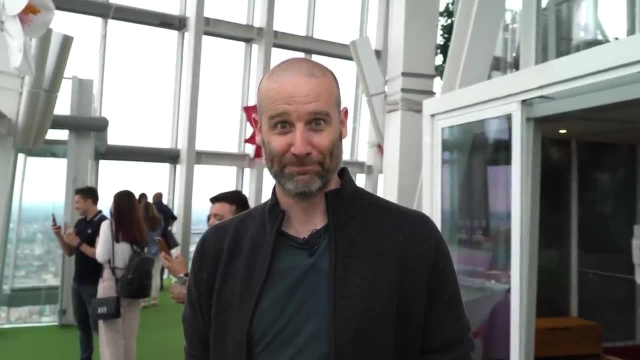 Did you really climb all the way to the top? Obviously I did. All right, let's go into the window. Fun fact: despite me trying to do this properly, the security at the Shard won't let any random visitor use the stairs, because they're trying. 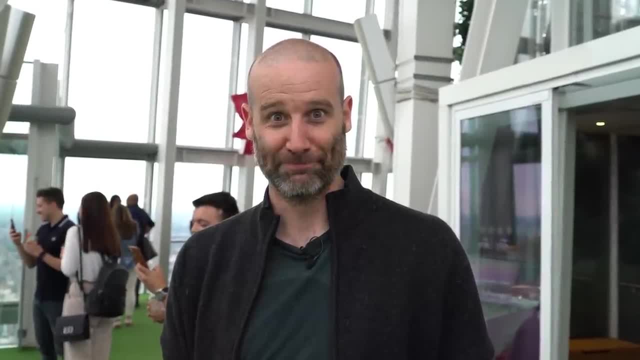 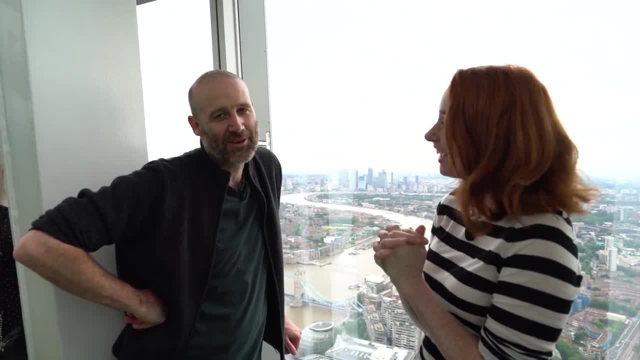 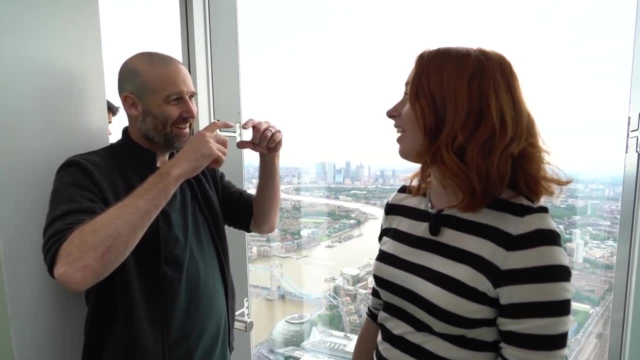 although, speaking of the Shard security, how's your plan going? Yeah, I don't know if you noticed, but we no longer have any geometric equipment with us. You know what? I nearly bought a tiny protractor. I think we got stopped. 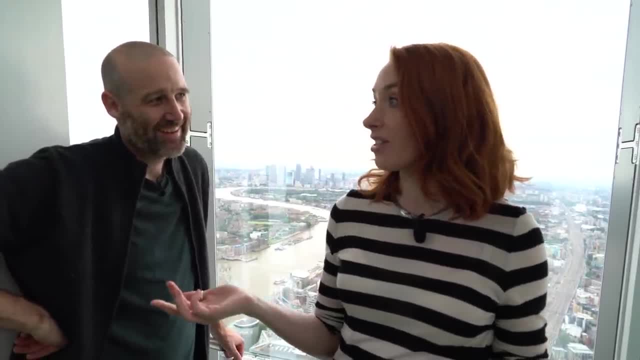 The thing is, I think it was my fancy-pants laser driven inclinometer. I think it was the inclinometer, I think that was the thing They said. it could have been used as a weapon, which I mean I was like what about this? 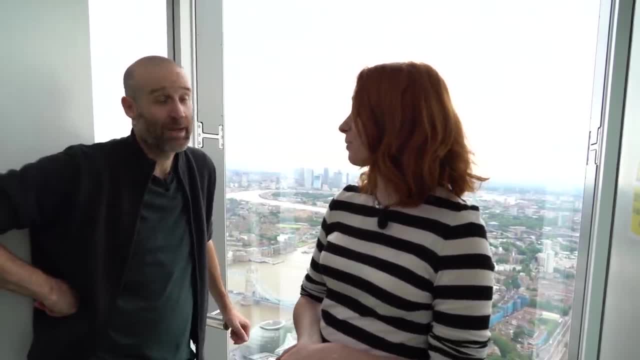 And they're like: oh no, that's definitely a weapon. That's how I feel about maths. is that it can be used as a weapon? Yeah, it's going to be used as a weapon. So we're up at the top of the shard. 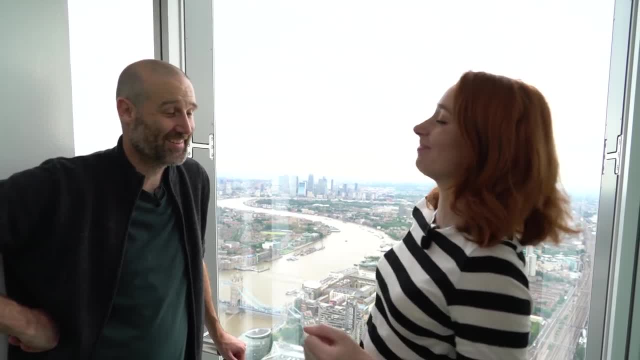 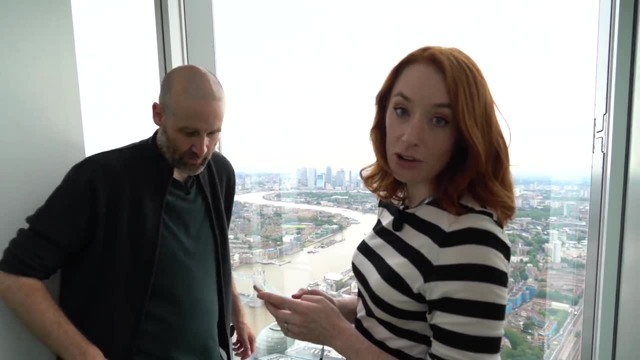 We've been promised a cocktail. They've confiscated our contraband Now so that Matt's video isn't completely ruined. it turns out that there is actually an app that you can get on your phone that does a similar thing. We've got these free guidebooks, so we're going to cobble together. 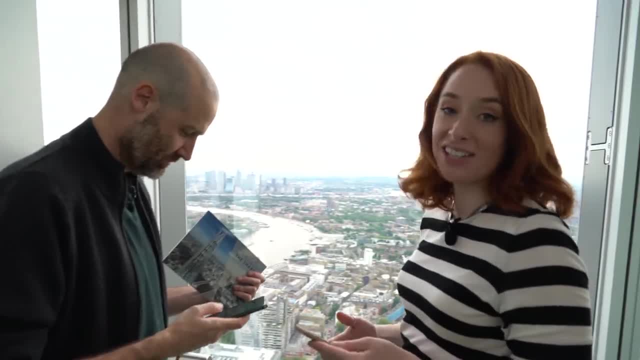 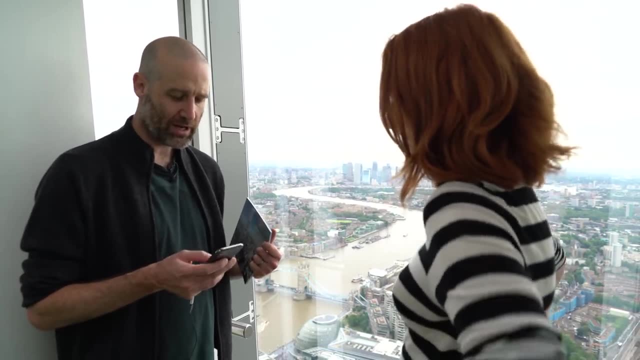 I'll tell you what Matt didn't have: health and safety like this in Alperoni's day. No one in the mountain going. you can't bring that astrolabe up here. It's got pointy brass edges. I'm running the inclinometer app on my iPhone. 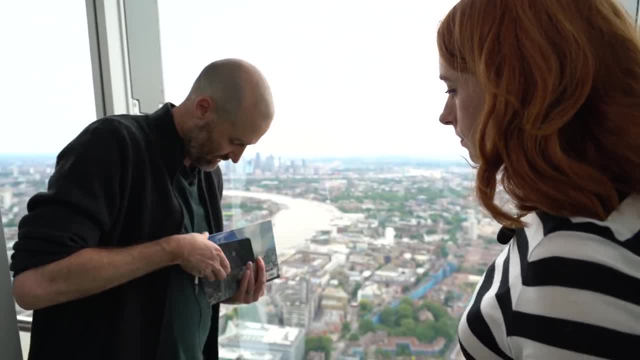 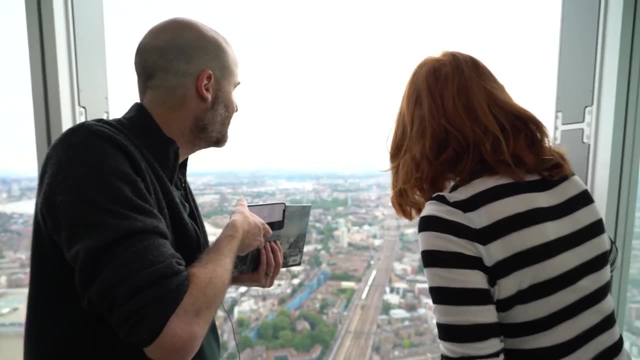 I think what we'll do is I'll put this on here like this, and then I'll try and use the shard. Where's the horizon? Is it like It's a bit mountain range over there, isn't it? It's a bit mountainy. 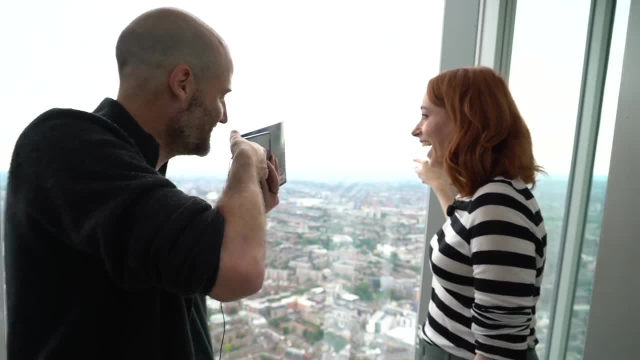 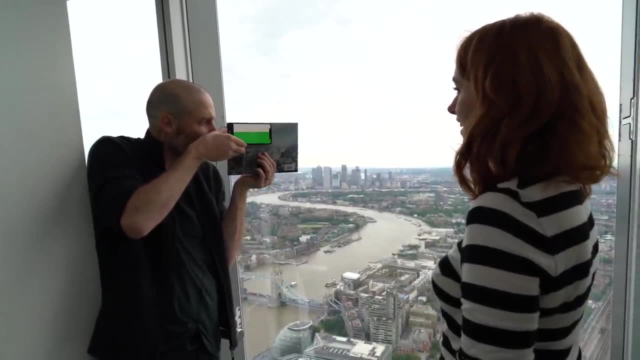 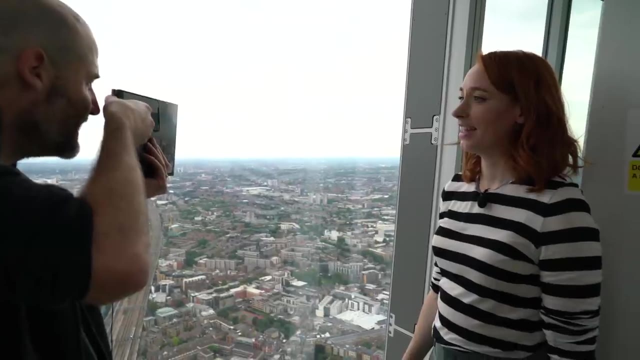 Top of the mountain, bottom of the mountain, Like there's going to be a difference. Okay, Hang on over. that way is a bit more flat. The book makes all the difference with this, Okay, so Okay, I reckon I'm looking at it now. 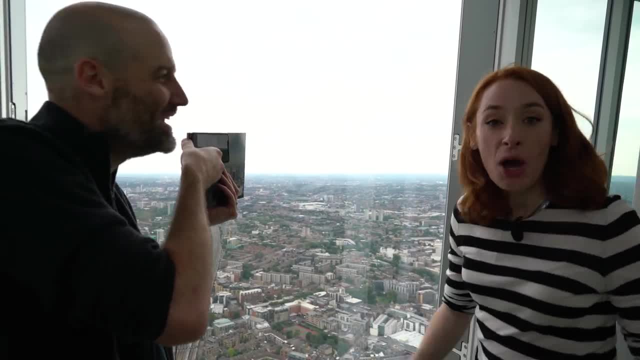 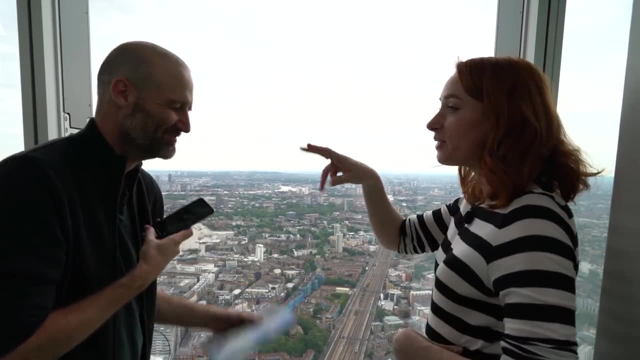 One degree One. We need decimal places on this app. Wait, it doesn't do sub-degree between zero and one degree. It was flickering between one and two. Should we go? one and a half? It's close to two. It's quite close to two. 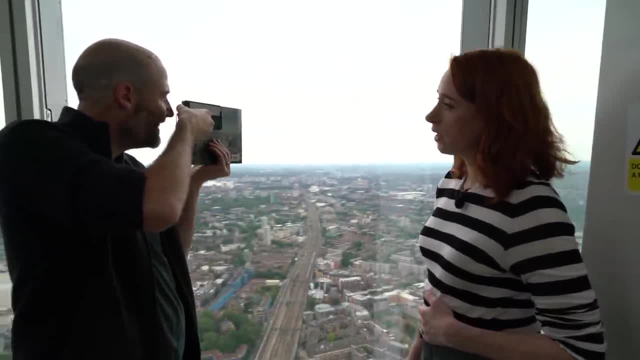 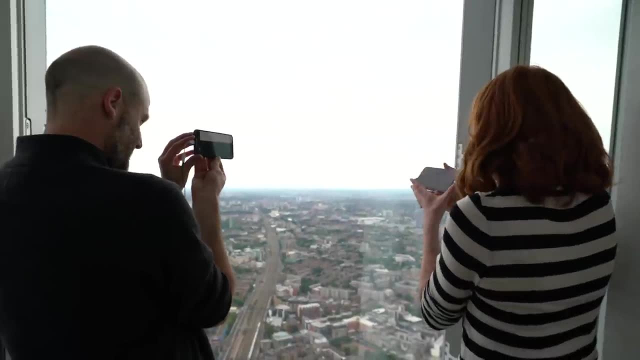 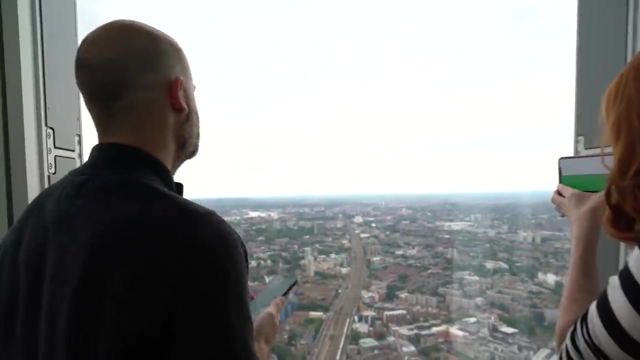 Here I go, Let's go 1.8.. Three degrees, Really, Yeah. So we're saying what? between somewhere between one and three degrees, depending on Two, I reckon one and a half, Yeah, One. 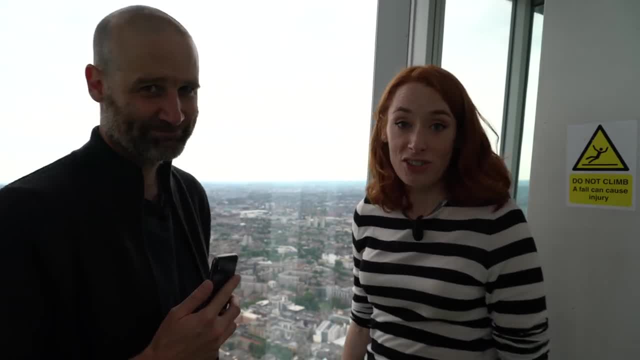 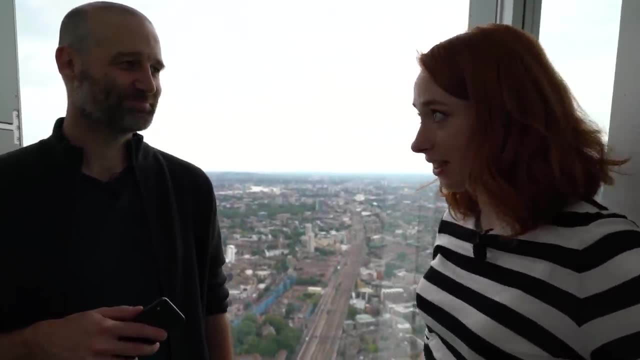 What's our consensus? Our consensus is Matt and I shouldn't do scientific experiments. No, Look, I revised my original expectation that we would get within a thousand kilometres, if that's any help. Now between 10 and 10 million, I'm very happy with. 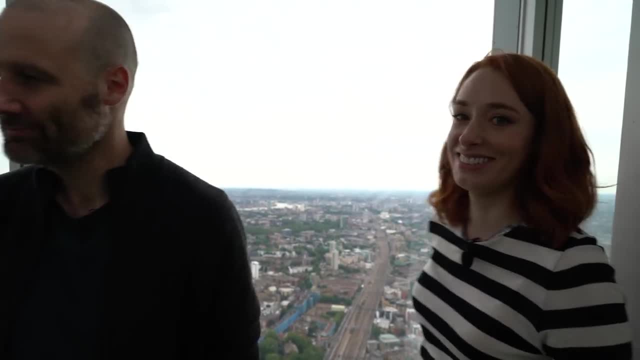 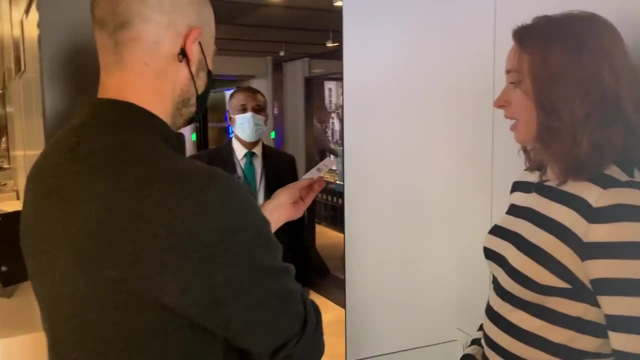 Exactly, I think we're. So we're going to get a cocktail, Let's get a cocktail. The cocktail is compulsory. It comes with a ticket. We can't opt out. What is it? Good question: A protractor. A protractor. 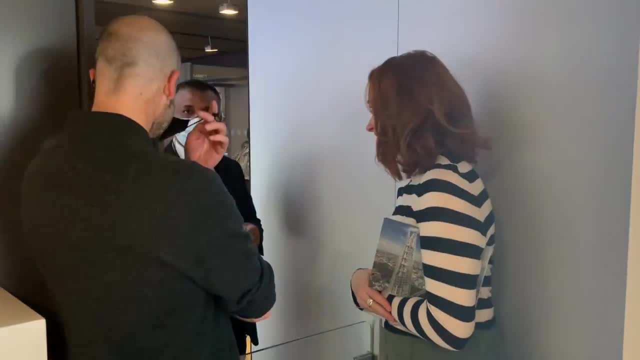 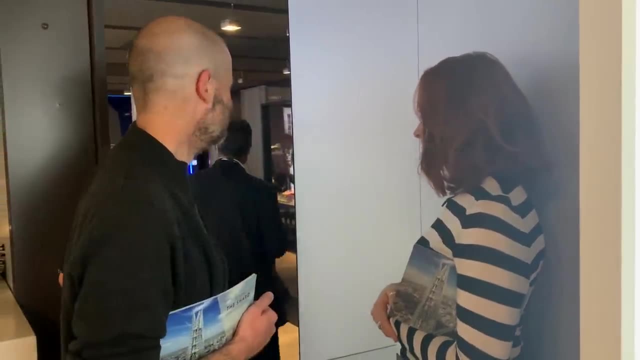 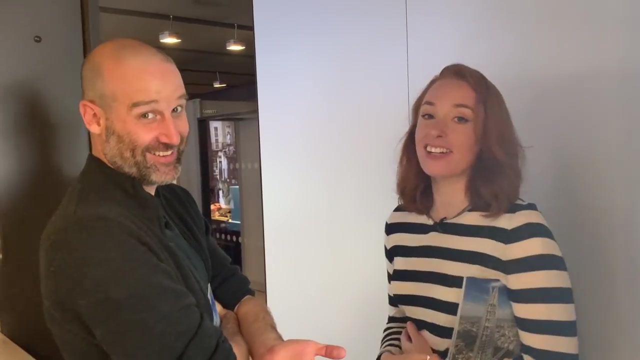 A protractor, Yeah, And a spirit level And a dynamometer, Oh, okay. Okay, I'll see if I can find it. I mean, it's very obviously a protractor. I'll just see if I can find it in amongst all the. 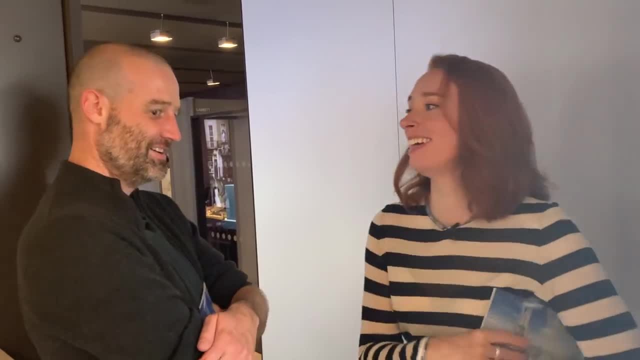 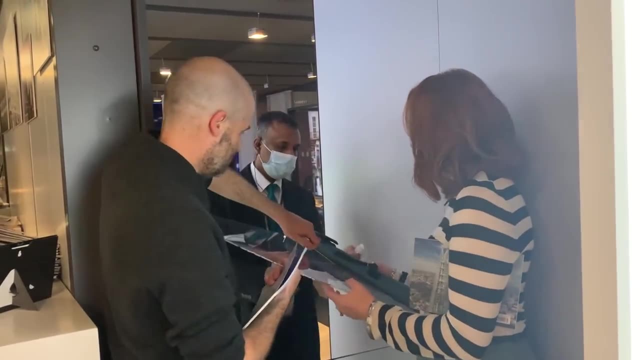 No, I have to say that'll be in the geometry bin. I don't know. Thank you very much. Thank you so much. Thank you very much. That's my plumb line. It's all in a good working order. 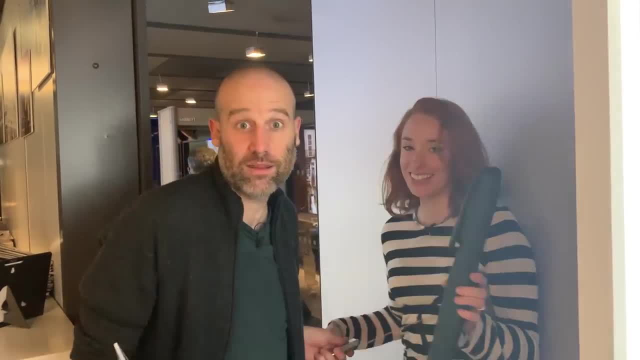 Is it all in working order? Let me check the. I'm not having any of that. We've tied the plumb line. Sense of humour, Sense of humour, failure. Okay, we're back, Having been reunited with our geometric equipment. 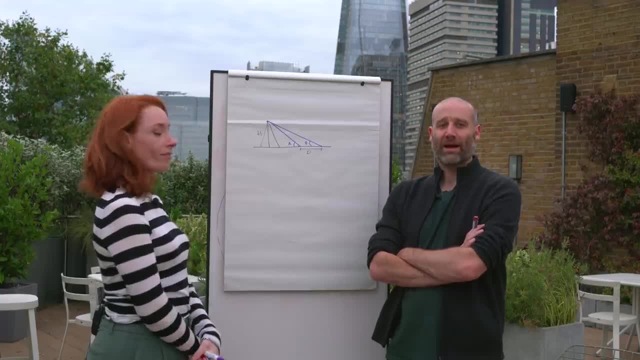 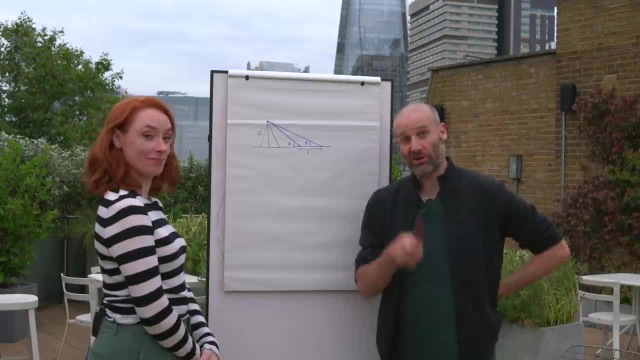 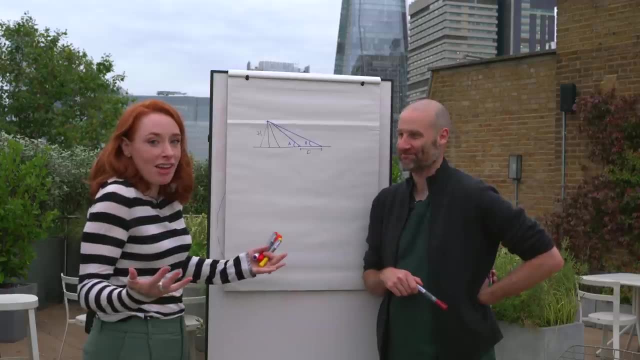 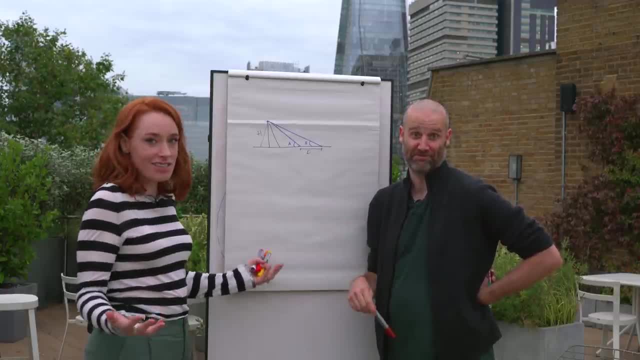 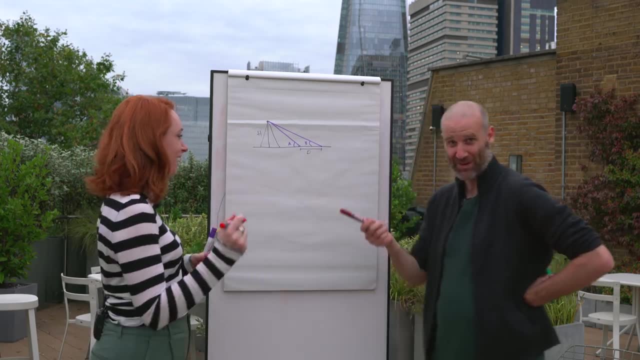 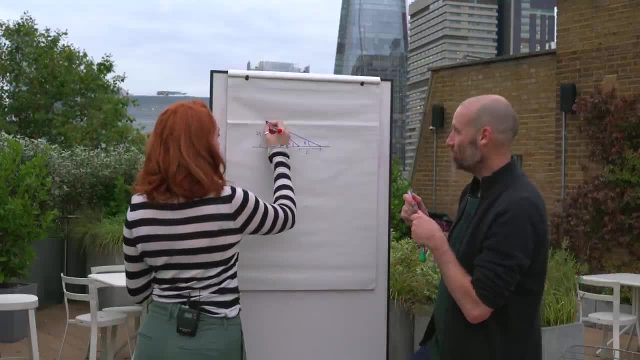 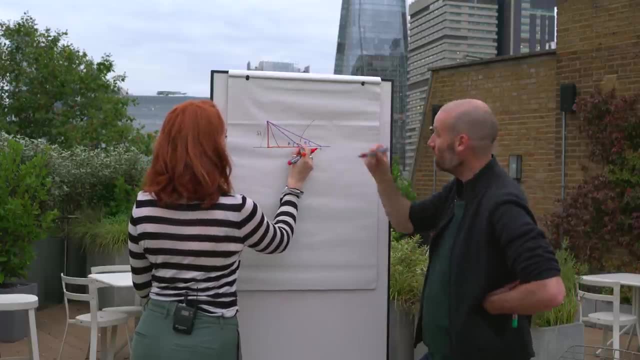 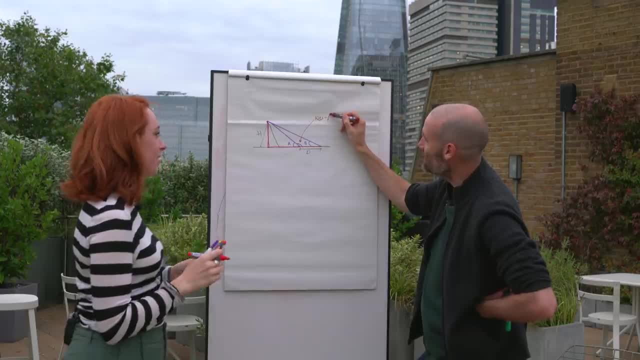 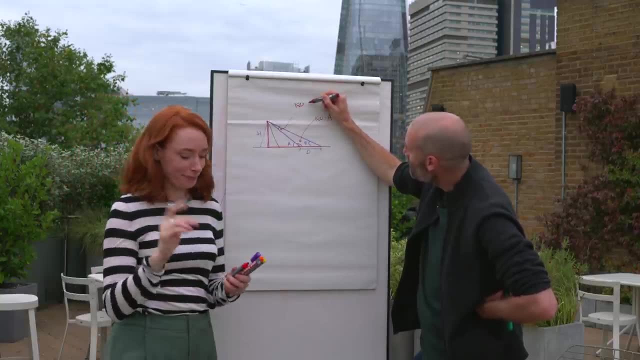 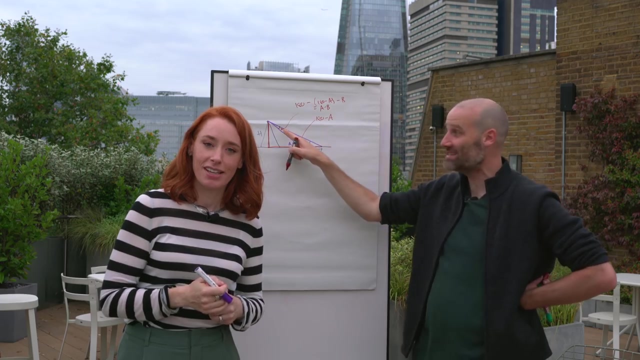 that angle in, there is going to be one that's 180 minus a, which means this little angle up here. that one is 180 minus 180 minus a minus b, which equals a minus b. how nice is that, that little angle, do you think, you see? you see why time's better? because i don't need any of that, any of. 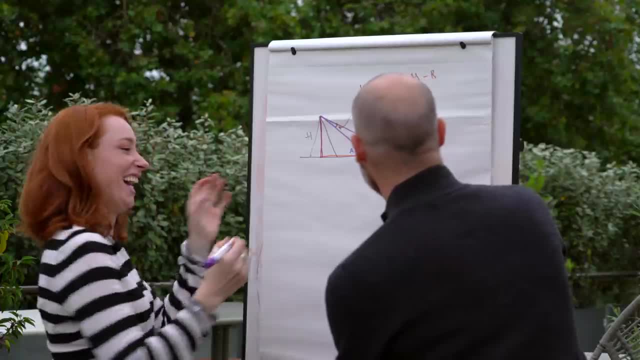 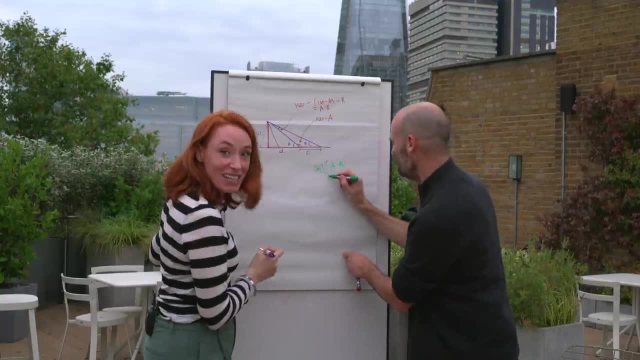 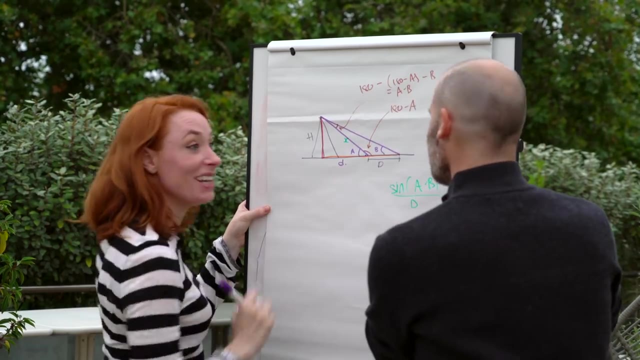 that okay and go okay. so, uh, if i do this, so we've got a minus. let's call this track that i'm doing the sign rule, so opposite. that is actually really hard, it really is, uh. and then, okay, what are we calling this? we call this x, you can call it whatever you like. oh, really, i don't need it. 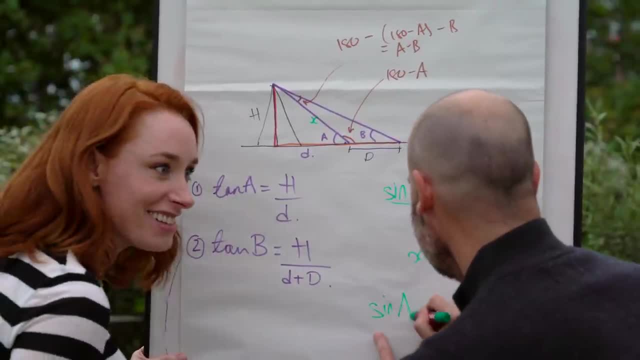 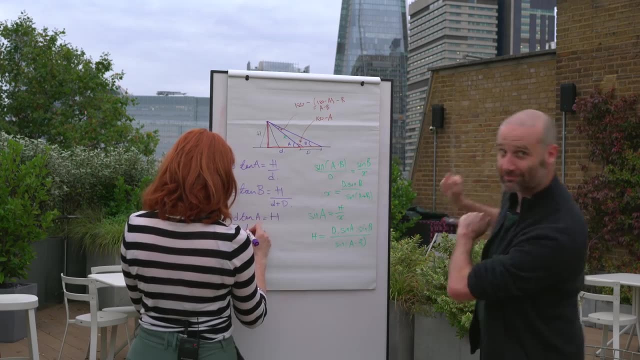 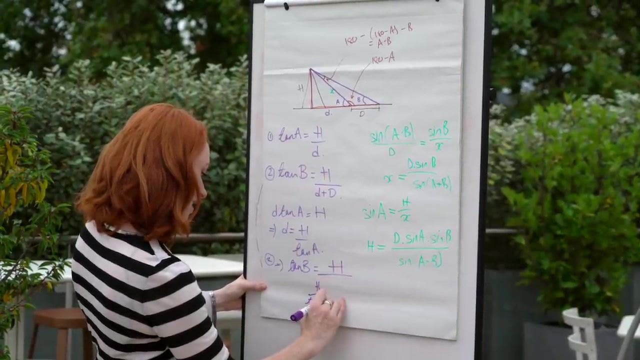 i know everything, but i don't know a little d. it's not a race. oh yes, it is times a. sign of b. i'm not distracting you and you are completely. so this means that it's about who gets it right not to get the quickest. so over tan a plus d. 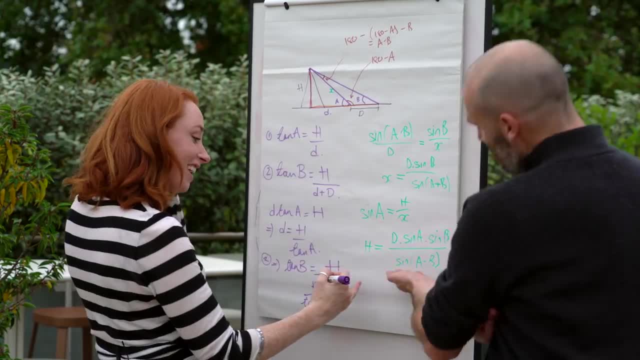 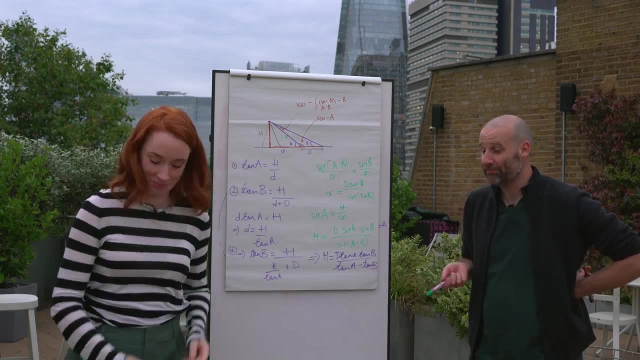 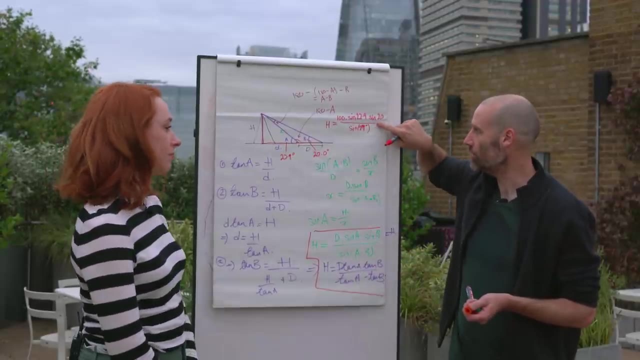 is this? look at this guy. i need your side, i need your side. very welcome, nice, pretty similar. yeah, i'm just a big sign fan, i'm gonna. oh, now i looked into this because like how on earth was this worked out? how did al um baruni do this? and they had look up, they had like tables, what for signs? 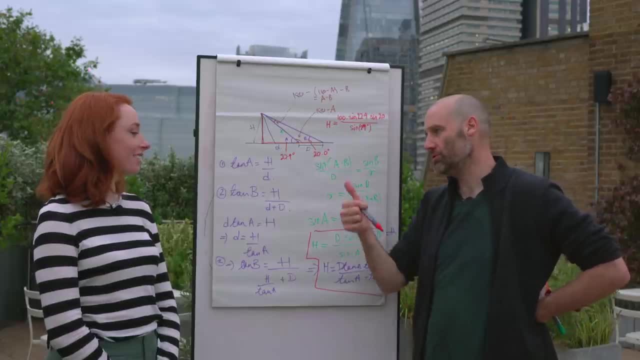 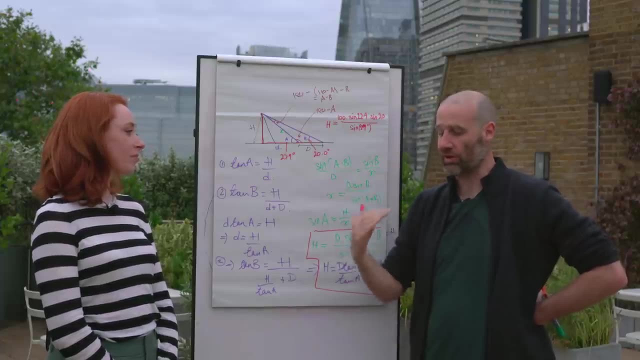 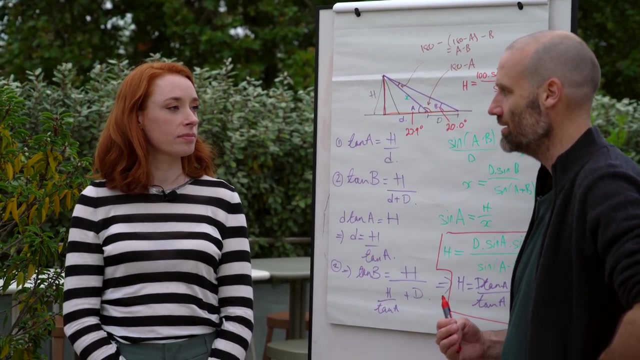 i don't know. oh, probably they had cords. they used cords a lot because of the greeks, apparently, and they genuinely had like just tables that have been pre-crunched for signs where people admitted it. i don't know how they did it, because it's pre-log and pre like infinite series or something. 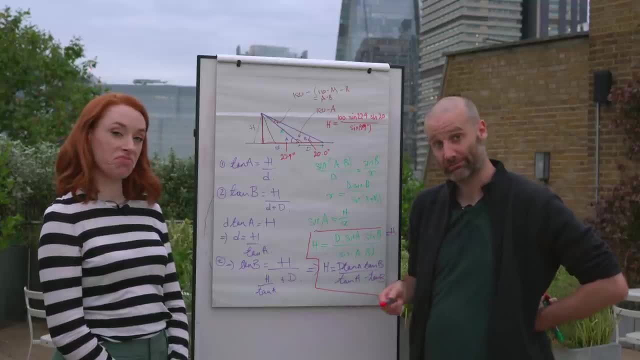 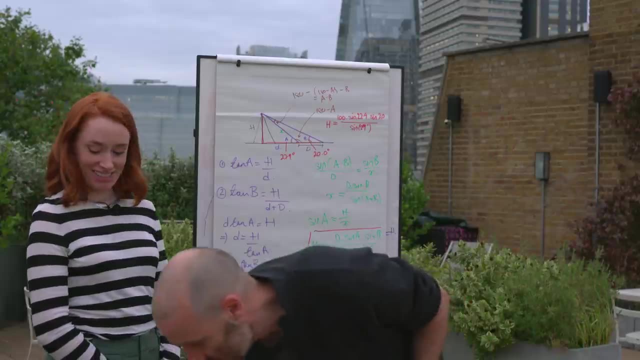 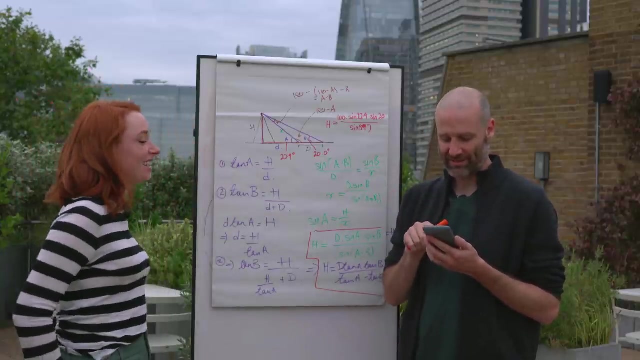 right, isn't it? so they must have looked into that. but that was getting cut. what i'm going to do, which i think is legit, is: um, i'm going to hand over to my assistant- you're electronic, because i'm pretty sure, as we established, he had an assistant and all this is. 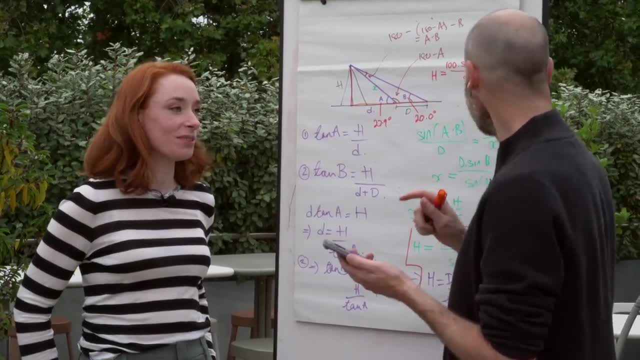 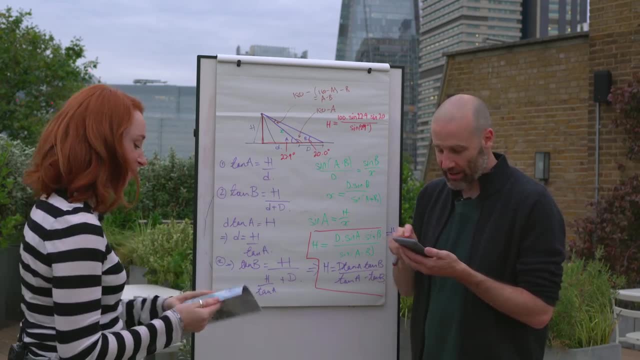 going to do is save me looking them up. okay, go on. okay, so here we go. uh, so, while you're doing that, do you want to do you want to? i'm just, i'm just going to look it up in the brochure. oh, okay, okay, you do you? look at me. 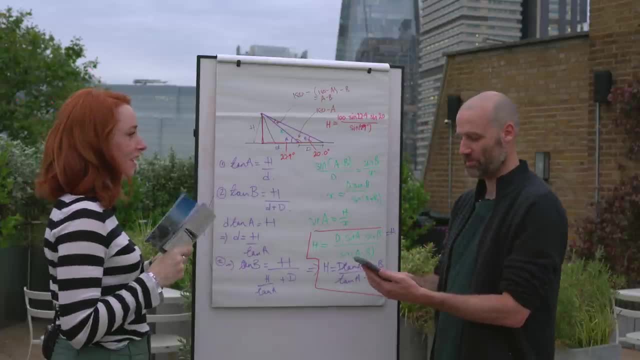 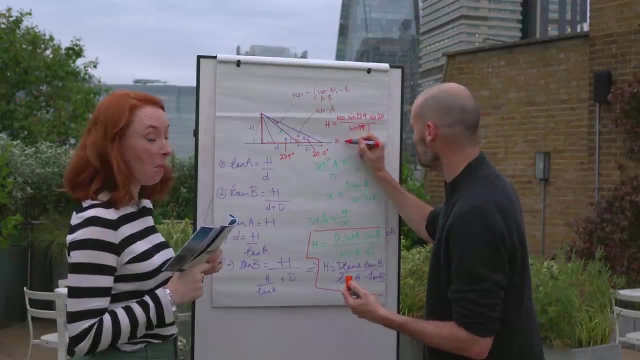 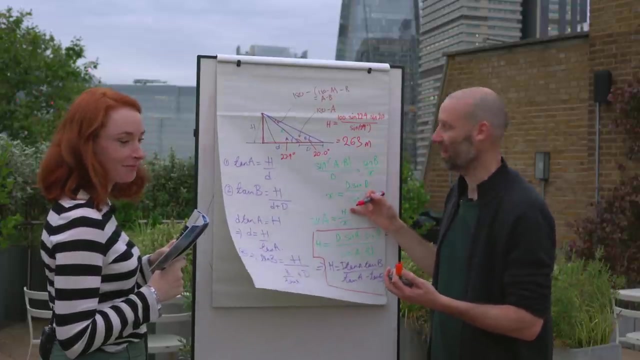 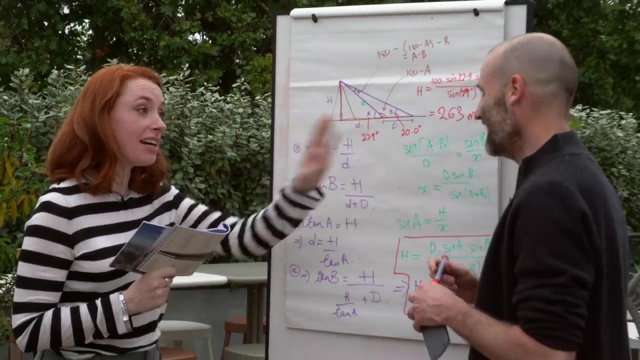 of two, i get this to be equals 263 metres n. please. thank you v One: i don't think i don't think i deserve the point one. i don't think you need that. okay, i mean honestly, though, actually, if you do that to one significant figure three times ten, to the two, yeah, 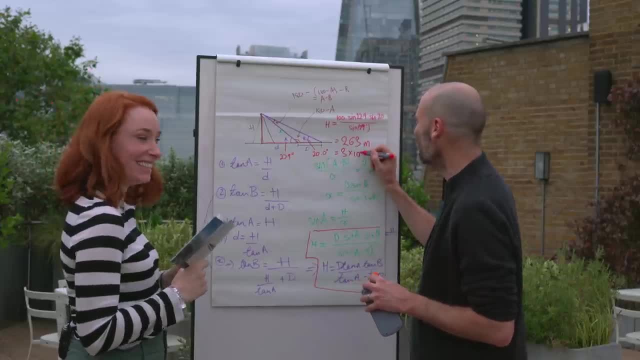 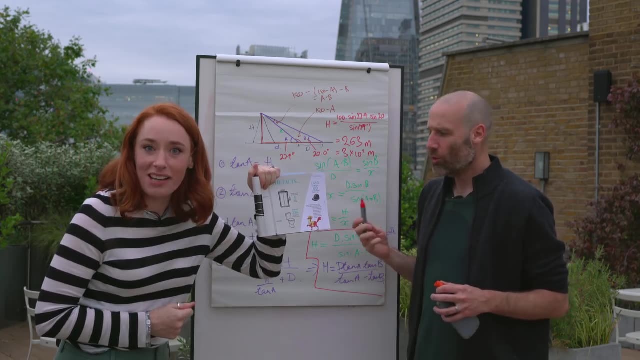 Yeah, you know what I'm picking up on what you're saying here. times 10 to the 2 metres- Oh my god, No way Is that right. 309 metres- Oh my goodness. Wait, is that the whole thing? or is that to the viewing platform? 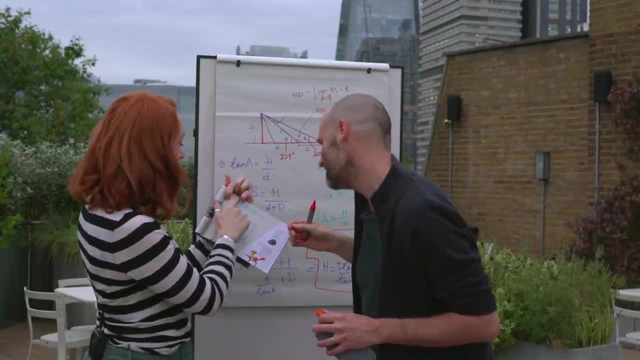 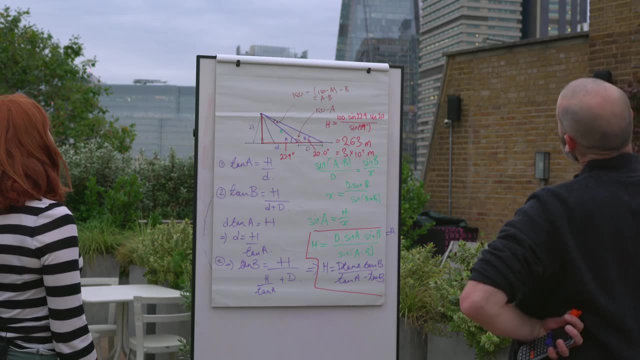 To the viewing platform, so it's probably 300.. No wait, so sorry, this is the whole thing. Yeah, yeah, yeah, so the viewing platform, I'm just eyeballing it. I would say that's maybe 37 metres. 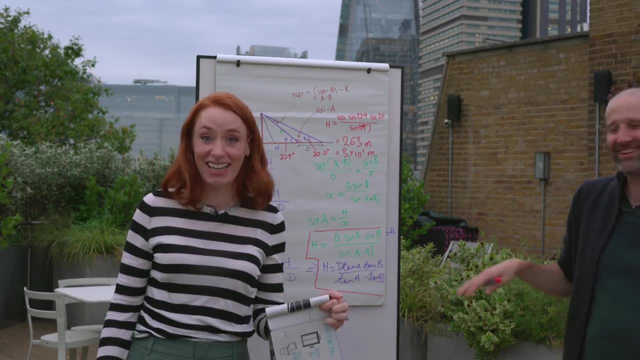 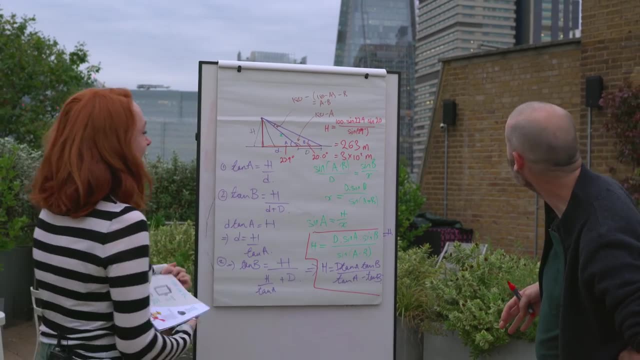 So, Oh, now you're eyeballing it. Was it 309?? After you made me walk down the street with your flippers, now he's eyeballing it. Sorry, 47 metres just from here, Okay, not bad. 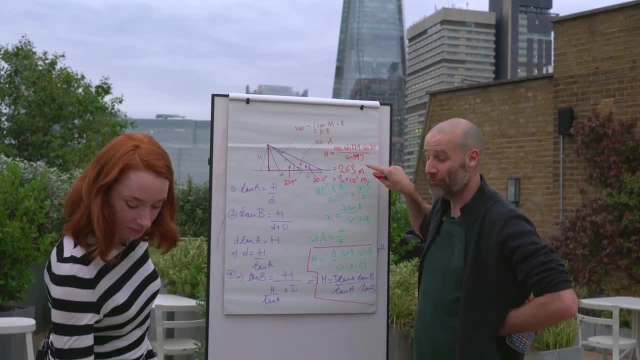 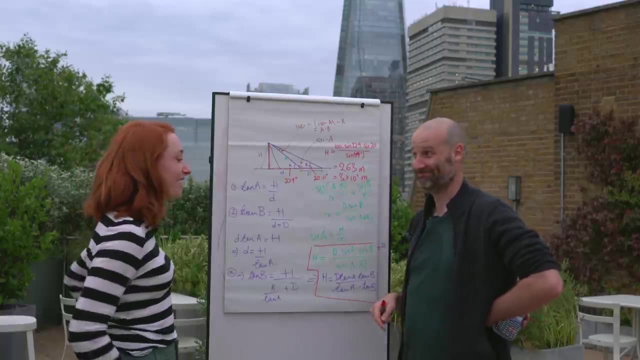 That's not bad. to be fair, Not bad. not bad For a bit of plastic I etched notches into and stupid shoes. It's not bad. It's within 15%. It's not bad. So this is where things started to go wrong. 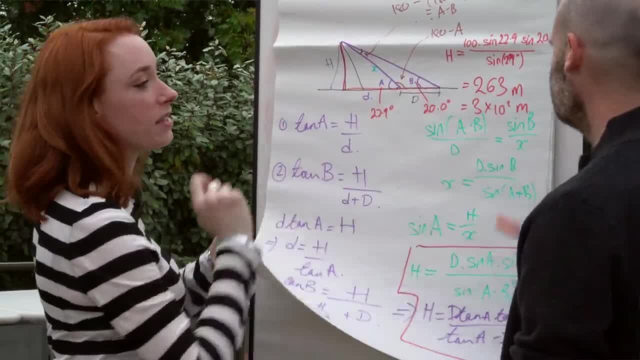 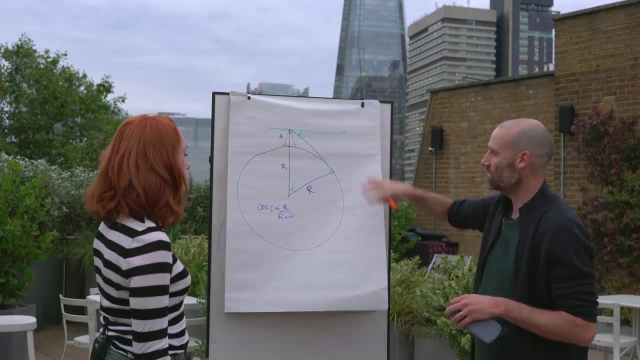 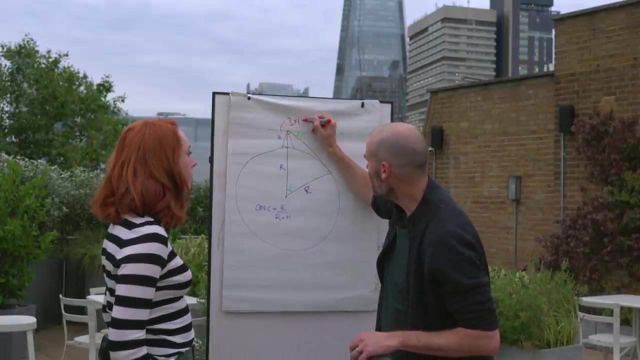 Oh, yeah, yeah, yeah. so then Let's use one significant figure. Okay, deal, deal. Okay, where's our picture of this? Okay, so, where's our earth? Bring it back over here. Okay, so we now know, and have verified, that our h here is 3 times 10 to the 2 metres. 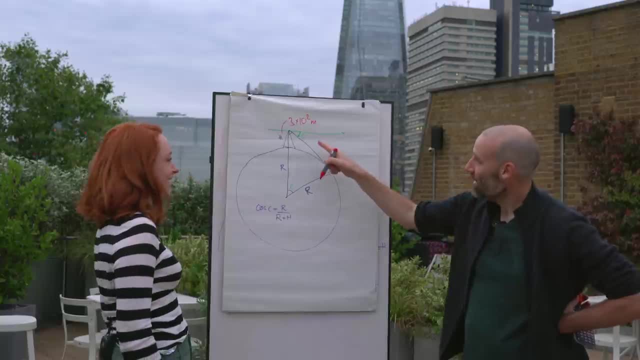 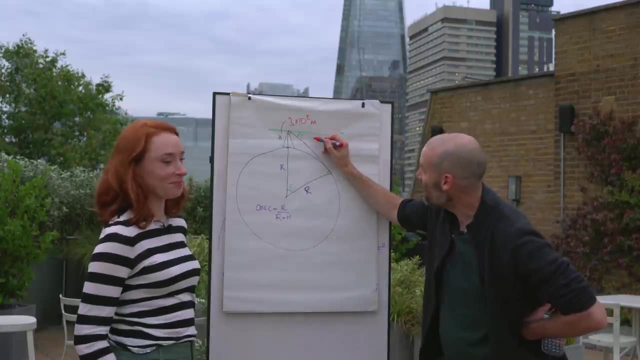 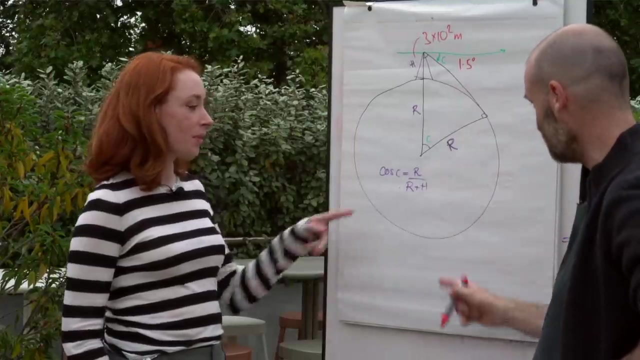 Or 300 for normal people. Now we agreed- non-ideal circumstances- that it's roughly 1.5 degrees that we were down. So how do we turn this into this With this little guy? Let's do it, Hang on. we've got to rearrange that to get r on its own. 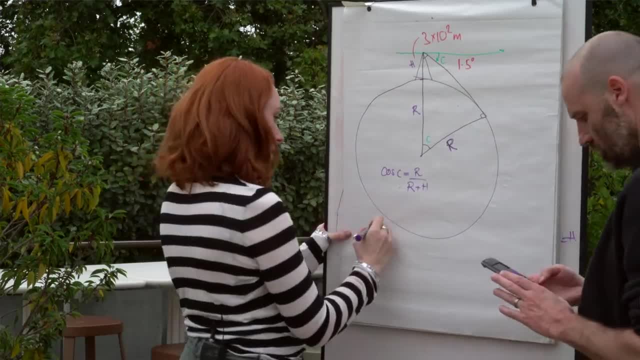 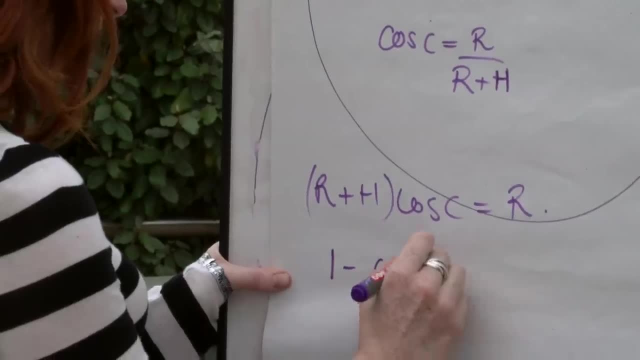 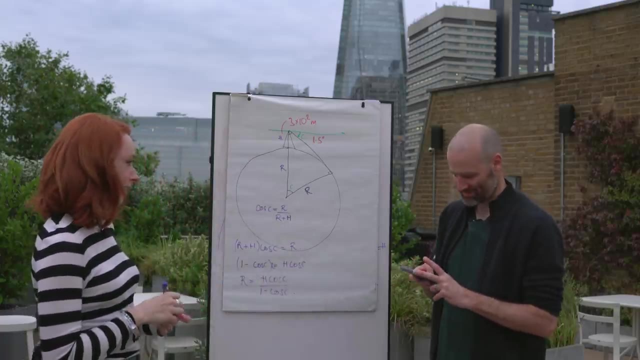 Do you want to rearrange Quick? there'll be a rearranging. sure, r plus h times cos c equals r One minus cos c, Yeah, and then you swing that underneath Yep, and then r is So 300 times the cosine of 1.5 degrees divided by. 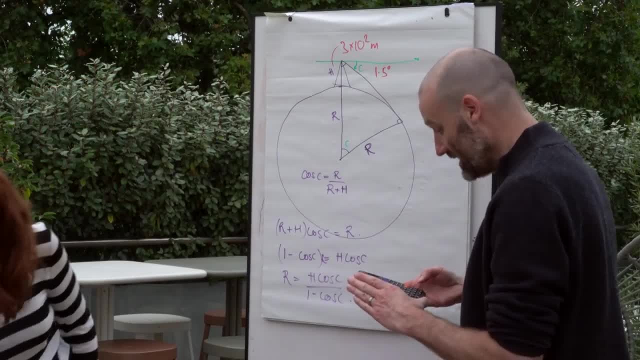 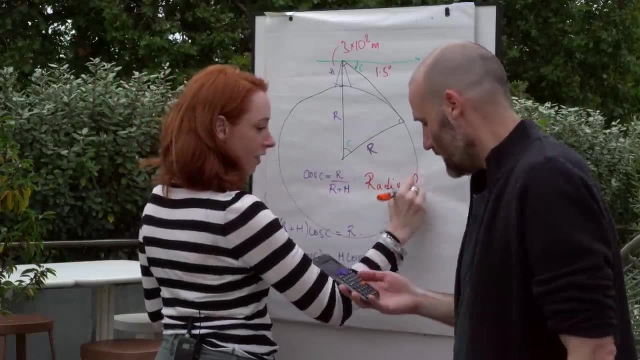 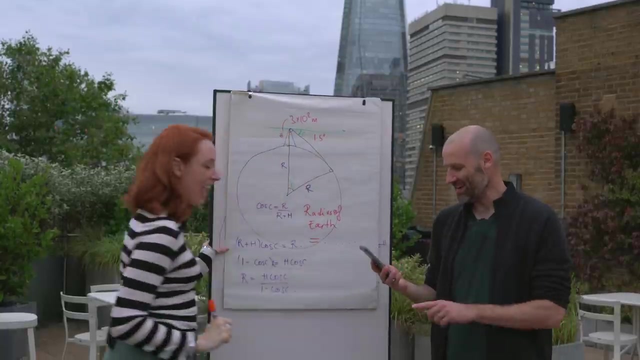 Divided by 1 minus the cosine of 1.5 degrees. Wait, I'm waiting. Oh, you're going to fill it in. Okay, I'm going to hit equals Ready? Yeah, It is. This is in metres. 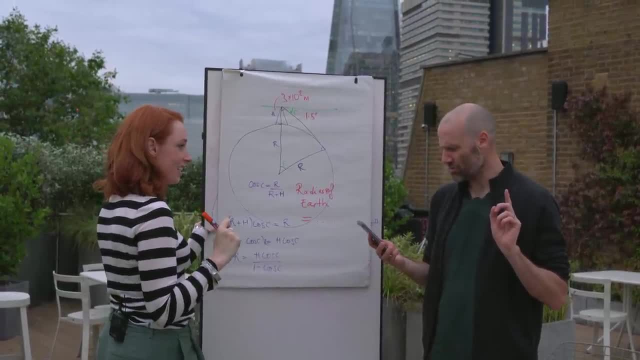 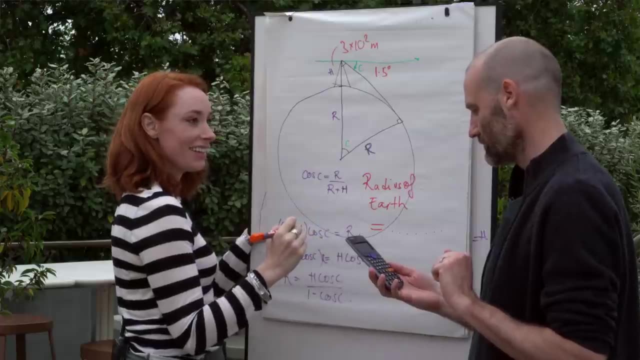 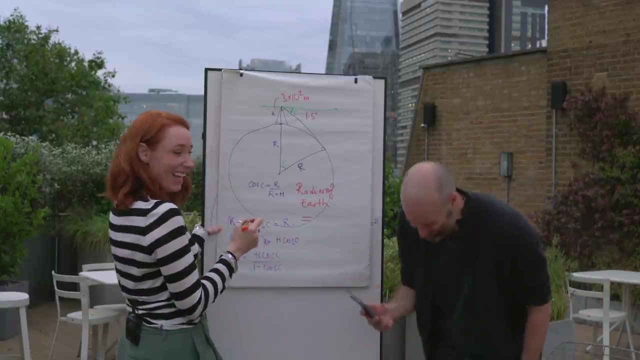 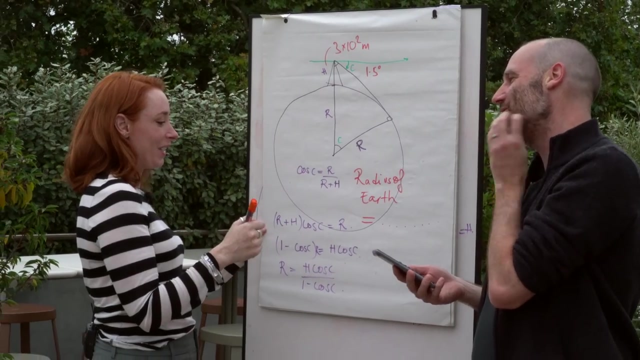 In metres. Should I switch to kilometres? Go on, give it to me in kilometres, Uh, 875.. Is that wrong? I think that's wrong. I think, Because it should be like 6,000, right, So we're out by an order of magnitude. 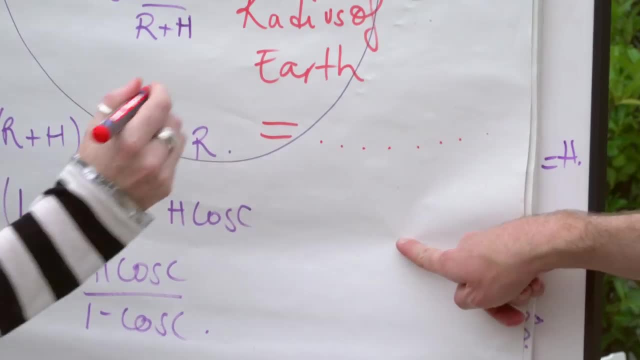 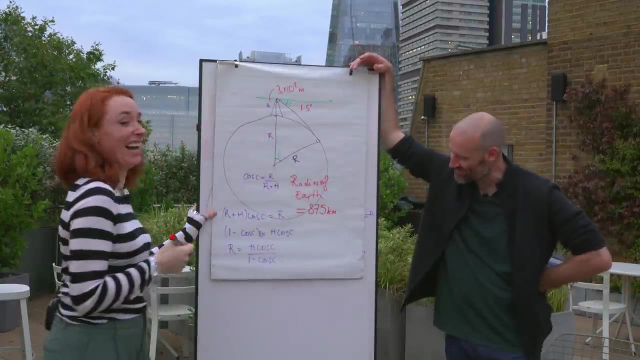 Oh no, Put it on the thing. 875k. There it is. You know what, Anna? It's a small world. It's a small world after all, Apparently. Wow, Wait, what is it? I think we've quite drastically. 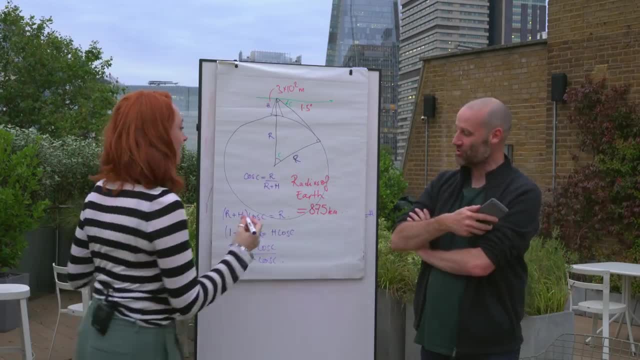 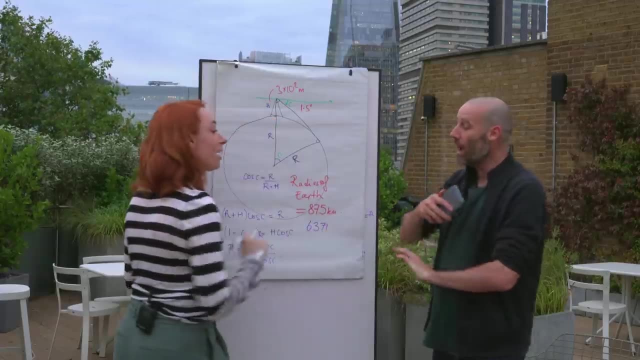 The real value. by the way, Yeah, yeah, yeah. What should it be? It's 6,371 kilometres, So I have my factor of 10.. If we rounded this to 1,000, it's the same order of magnitude. 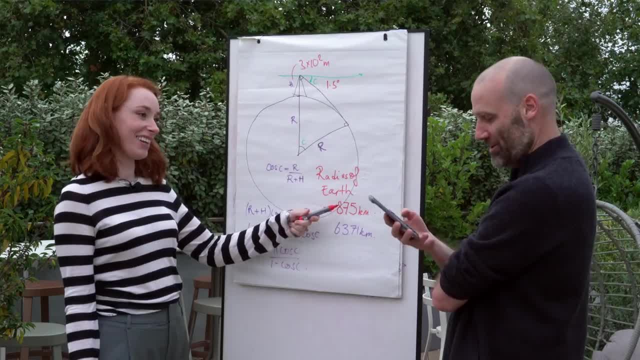 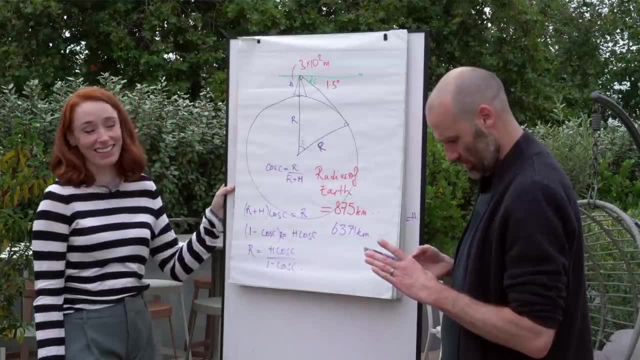 How big? Oh, Oh, Oh Oh. How big does that make the circumference of the earth? Wait, you're right, Give me a second. Uh, answer Times 2 times. Uh, where's my pie? Yeah, 5,500k. 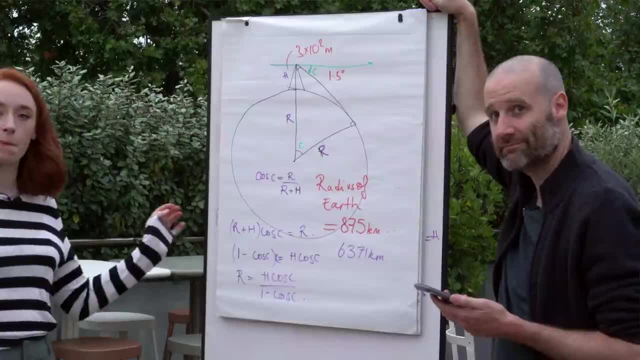 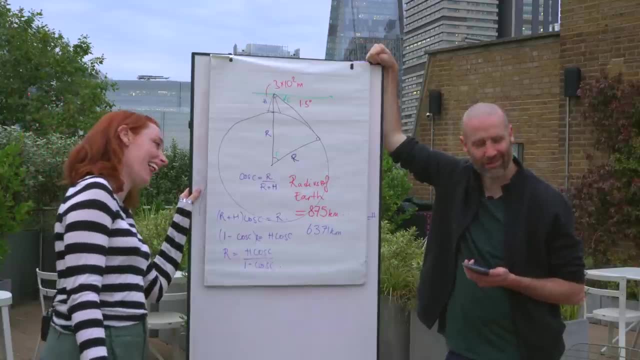 This is the circumference. It's also probably worth noting that your circumference is still smaller than the accurate radius. Oh, it's a little bigger. No, it's not 5,000.. No, Oh, you're right, you're right. 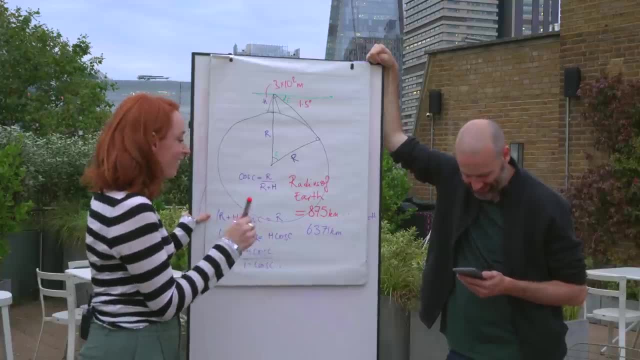 It's smaller. Oh God, What's the circumference? Okay, the circumference of our earth is 5,500k instead of 40. You know that song. I would walk 500 miles. That would be a tenth of the way around the earth. 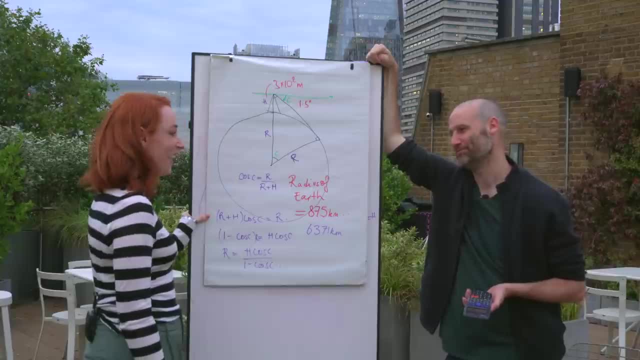 I am the opposite now of a flat-earther, I'm an extra-curvature-er. Not only is it a sphere, it's a really tight. Just a little bubble, Yeah, a little, little, little, little sphere. 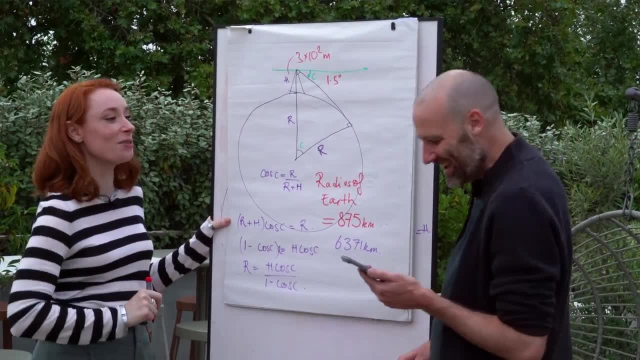 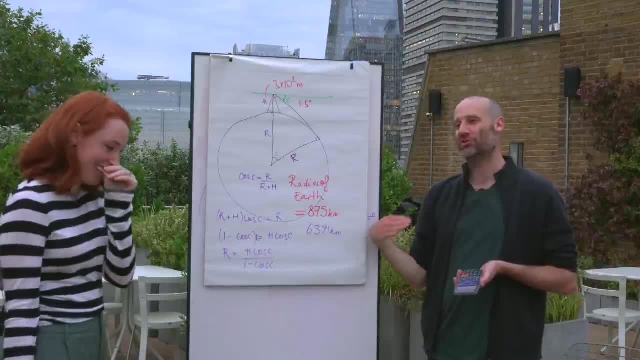 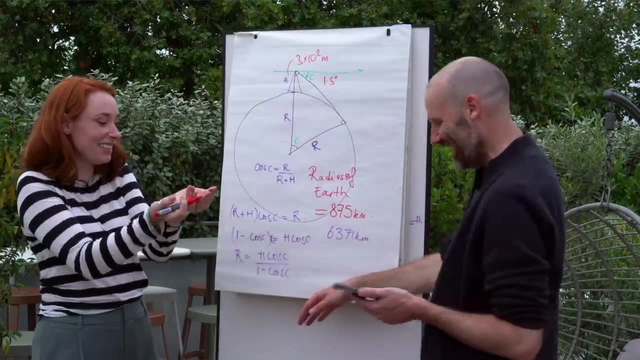 I am the opposite now of a flat-earther, I'm an extra-curvature-er. Not only is it a sphere, it's a really tight. Just a little bubble, Yeah, a little, little, little, little sphere. 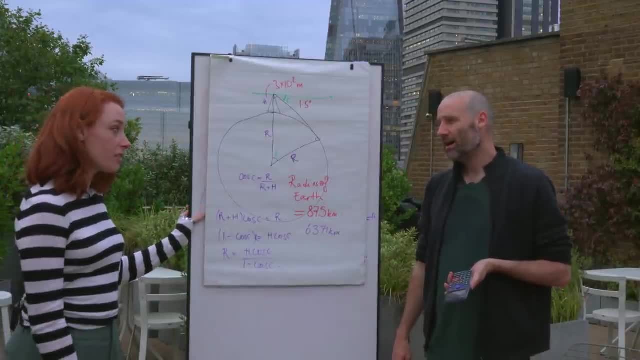 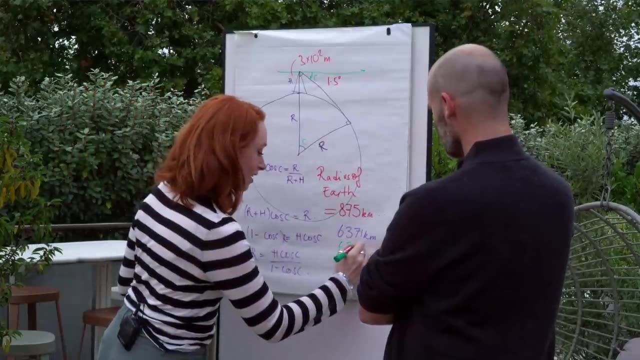 You know what? Don't feel too bad. Al Biroony got it under as well. Oh, okay, Yeah, he was under it, Maybe not quite as much as us. His number was 63, 22.. Oh, he's way off. 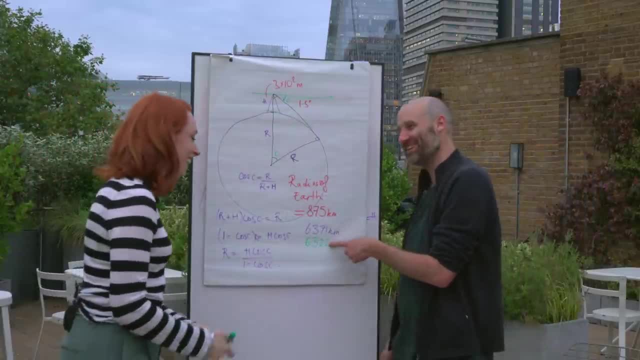 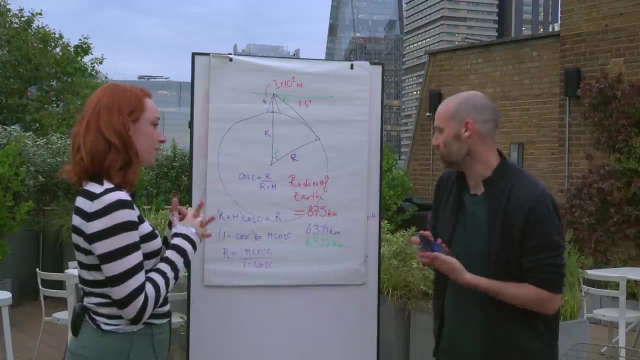 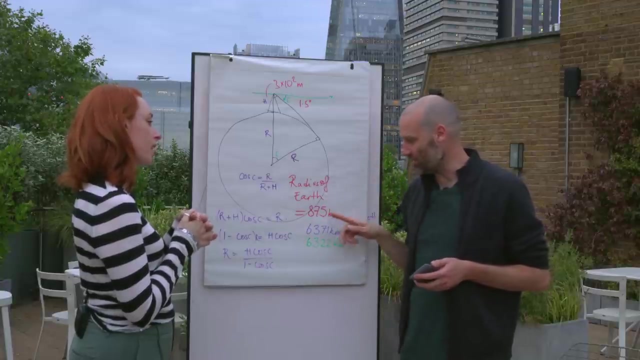 I mean, we're A thousand years ago. You know what You really are. You know what, If I'd been allowed my protractor, I think we would have because, to be honest, this just shows you how dependent on that angle it is. Because I think if we reverse, 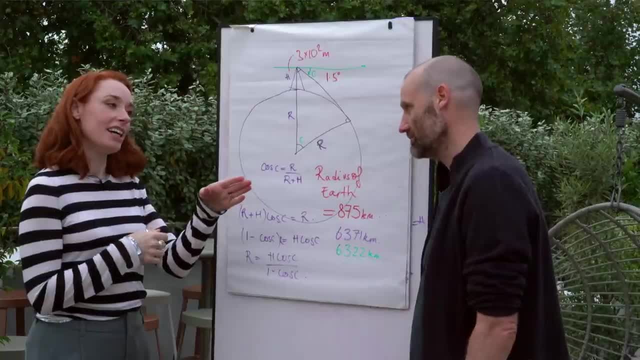 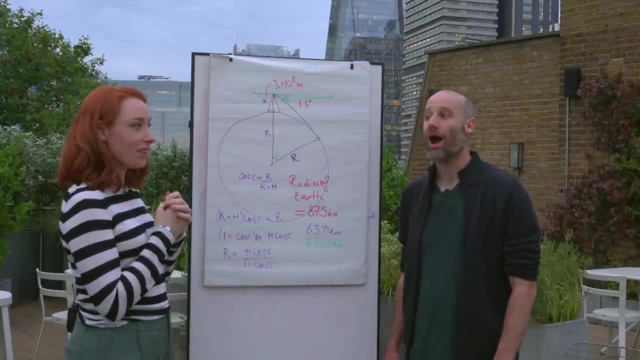 the number. It's like half a degree. It's like half a degree, Yeah, but I don't know if your protractor, brilliant as it was, as much as I loved the Perspex, I don't know if that could have given us half a degree. 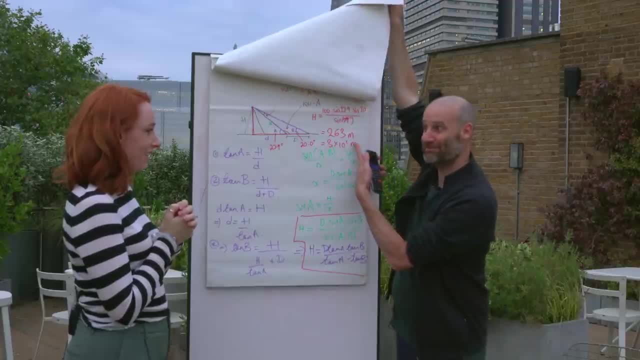 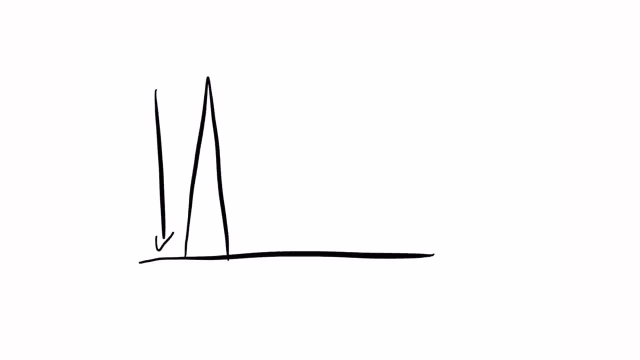 Yeah, but we got you know this was close For the record. while the Shard itself may be 309 metres top to bottom, the observation platform about here- that I looked it up afterwards- is only 243 metres. So when I calculated 263 compared to the actual height of the platform, I was only 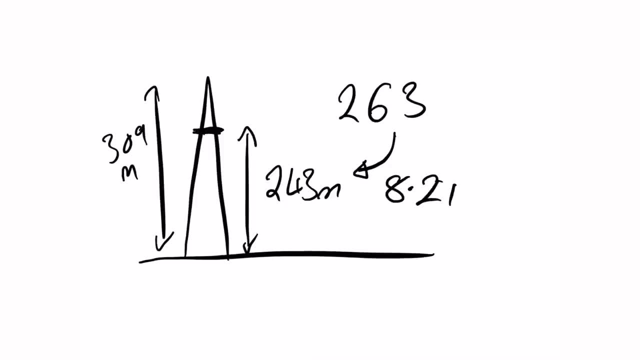 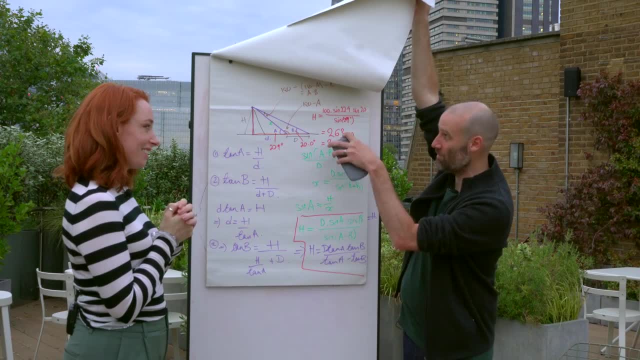 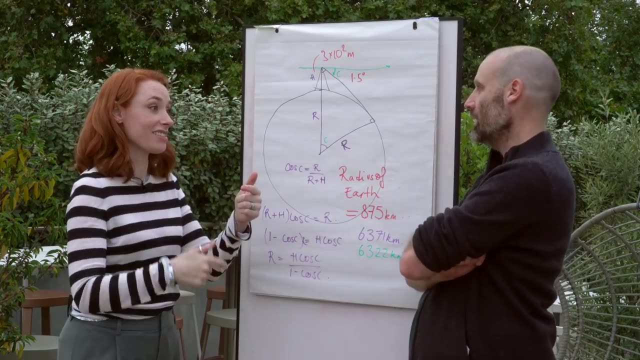 off by like 8.2%, which might be more luck than skill, but, for the record, not bad. We were measuring to point one of. Well, that's our big conclusion then, isn't it? Because maybe what you need to do is just use your qubits all the way around the earth. 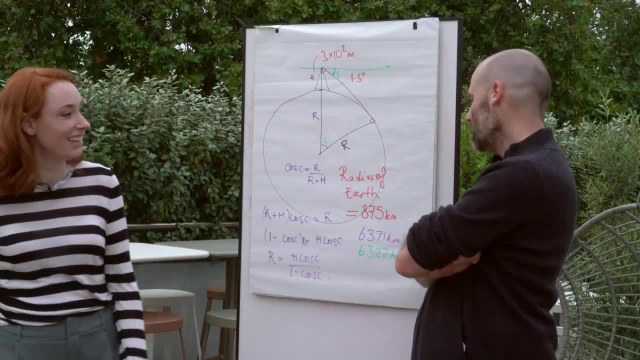 next time. Now you're talking Measure the whole, Okay, but the thing is we got a number and it's within an order of magnitude. It's not. It's not within an order of magnitude. It's not within an order of magnitude. 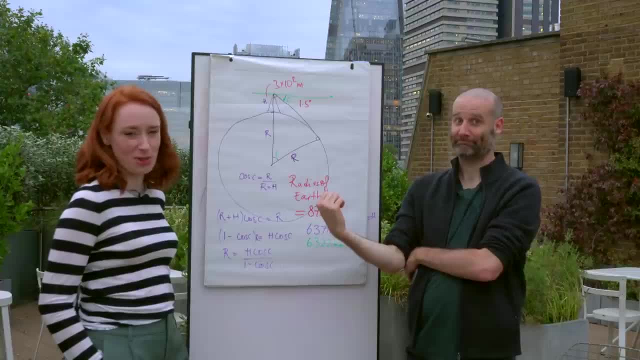 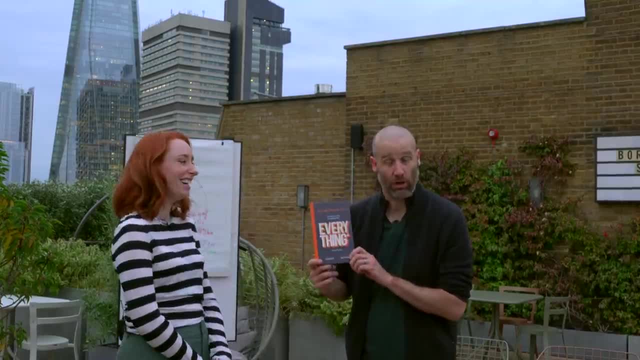 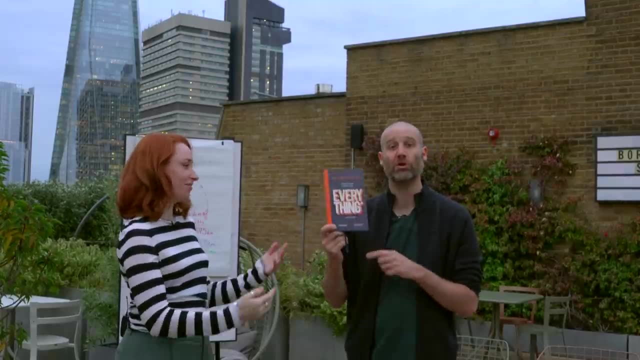 If you want to read the story of someone getting that right a millennium ago, you can get Rutherford and Fry's The Complete Guide to Absolutely Everything abridged. It's most but not everything. We couldn't fit absolutely everything in there, That's true. the book is finite, sadly.